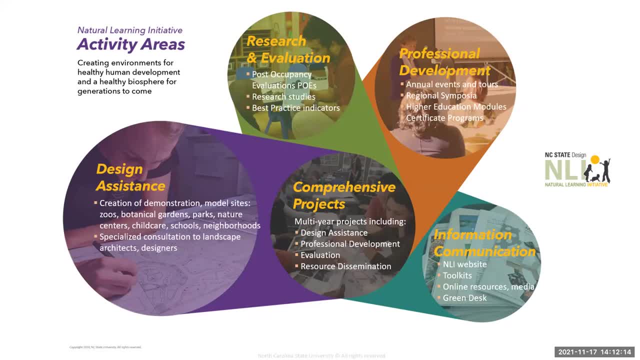 where we create demonstration or model sites, and that could be anywhere from at a child care center, a school, zoos, botanical gardens, parks or natural centers, And we help to naturalize the outdoor environment, incorporate more trees, more fruiting trees, vegetable gardening more. 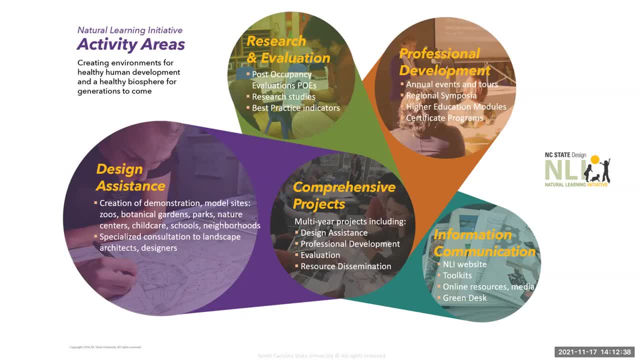 naturalized material, And then we have here on site specialized designers with backgrounds and landscape architecture to help design this space for our clientele. We also focus on research and evaluation and we have several different research studies that we're doing. We also have a lot of 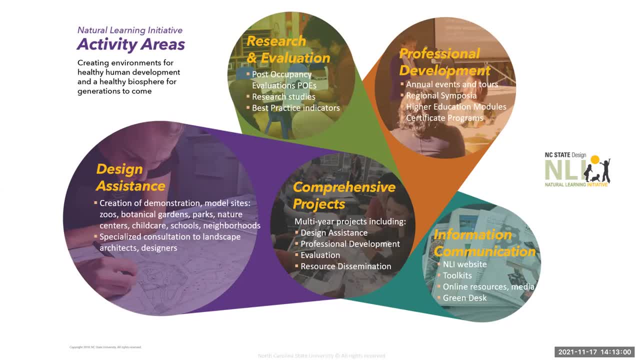 research that we're doing. We also have best practice indicators. We also have a section on professional development where we have annual events tours. We also have online distance learning and I'll highlight this a little bit more, but we have two certificate courses that we 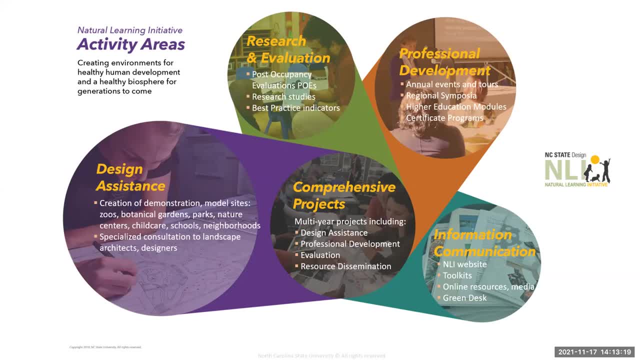 do each year. We also do information communication. So our website and we are constantly updating and adding new information and material. We have our toolkit, We have, as I said, online resources, and then we have various videos along with that and our green desk And, lastly, we have comprehensive projects which are mainly 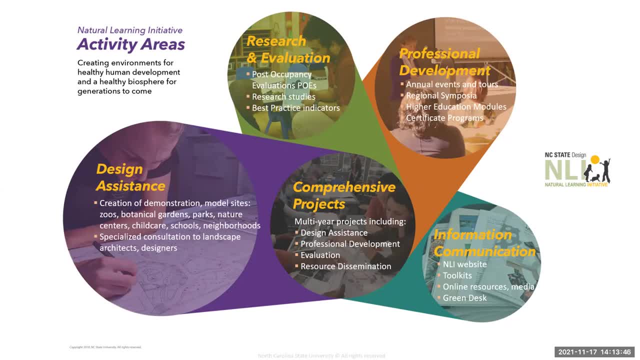 multi-year projects that include design assistance, evaluation of the outdoor learning environment, professional development opportunities and then resource dissemination. So in our garden we have a lot of resources, We have a lot of resources, We have materials and resources, We have our toolkit, We have, as I said, online resources and then we have various videos. 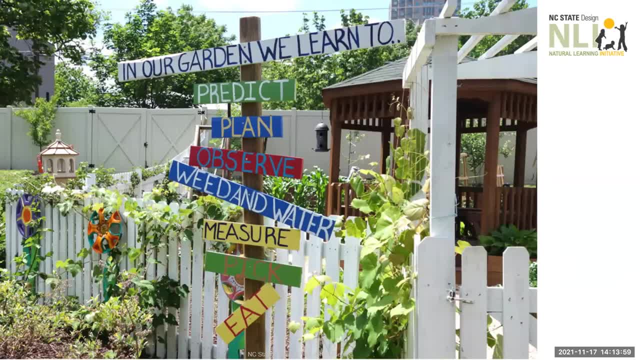 that we can share with you. So in our garden we are able to learn. our children are able to learn and predict, plan, observe, nurture the fruits and vegetable in the gardens that they are being able to participate in, measure the maturity of different fruits and vegetables or plants in the garden. 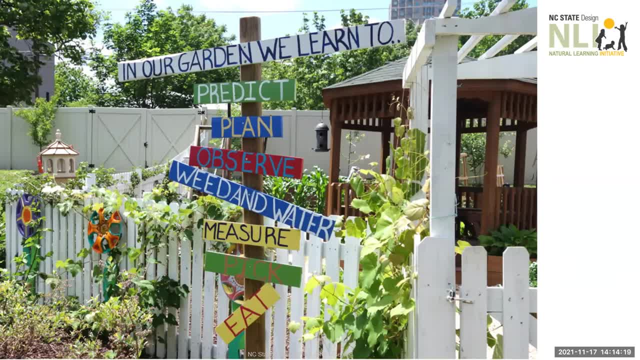 harvest and then eat at the end of that garden cycle for that particular plant, So they are able to try different fruits and vegetables that they may have not ever tried before. So we have a lot of resources. We have a lot of resources that they may have not ever had the opportunity to do so. 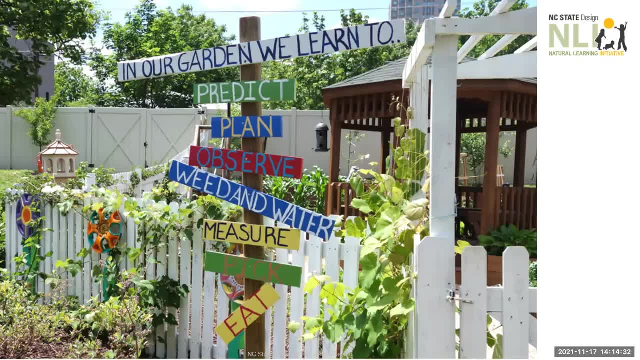 And then they also are able to learn where their fruits and vegetables and other plants come from, versus going in a store and going with their mother or father or a guardian and buying things at the store, That they're able to learn that it actually grows outside in their garden. 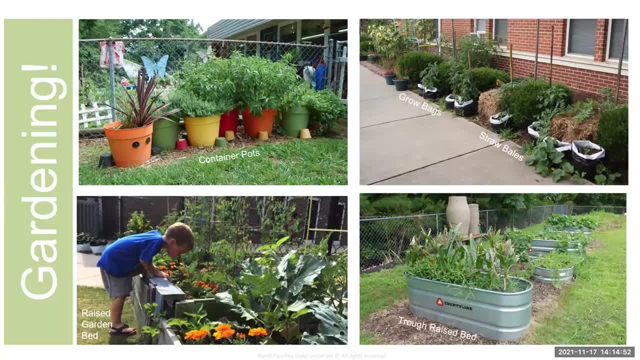 So working, especially with young children, when you're having a garden, it doesn't have to be this big in-ground or this nice laid out raised garden area. We at the National Learning Initiative like to incorporate things that might already be at the center, or it could be something that's very 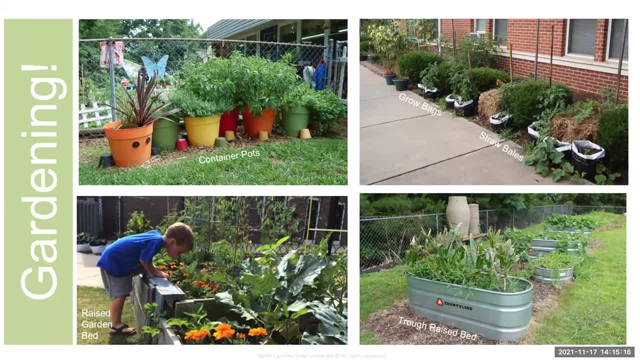 inexpensive and it's easy to create different gardening areas. So here you can see, at the upper left-hand side of the page, our container pots that they have laid out in a way that looks like a caterpillar, But you can see that they have. they're growing herbs and different other plants. We also encourage garden. 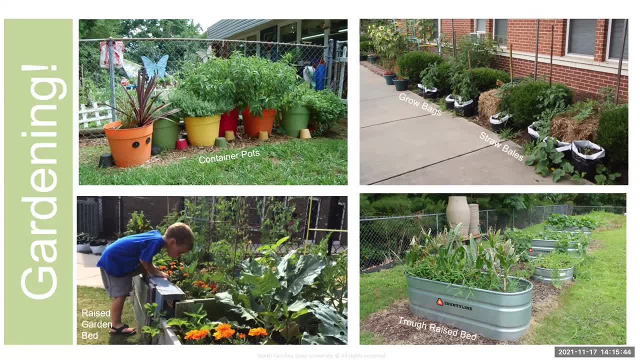 bit, I'm sorry. grow bags where you can find that, on Amazon or at your local hardware store, a home, like a Home Depot or Lowe's, which are very inexpensive and are easy to grow different fruits and vegetables. We also recommend straw bales which are like seasonal garden bed areas. 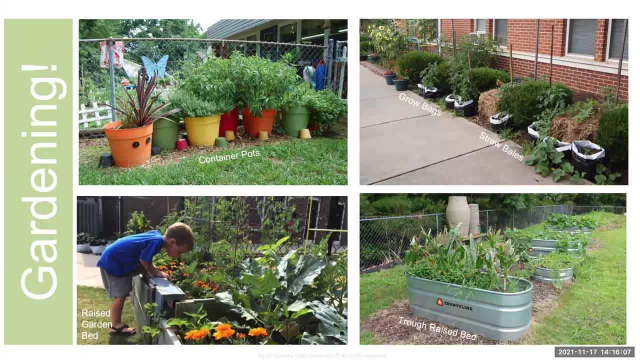 And this is a fun activity that children can participate in. They can help the teacher or the adult who is coming to educate children about gardening. They can participate by digging out all the loose straws and maybe later on composting those parts that can be added back. 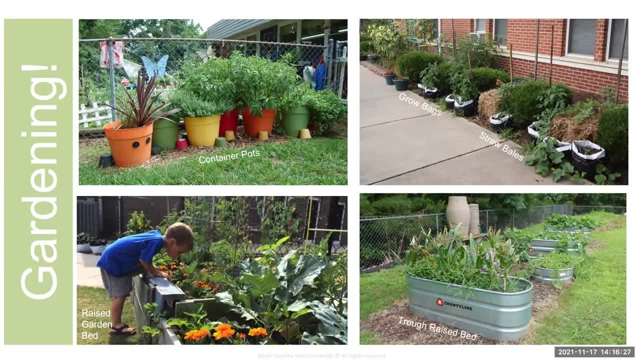 into the garden in a different way- gardening season, and then they can also help by planting those fruits and vegetables or flowers in the straw bales. We also recommend these raised beds down below here, trogs, which are fairly inexpensive and easy to maintain and at a height level that children can easily access. 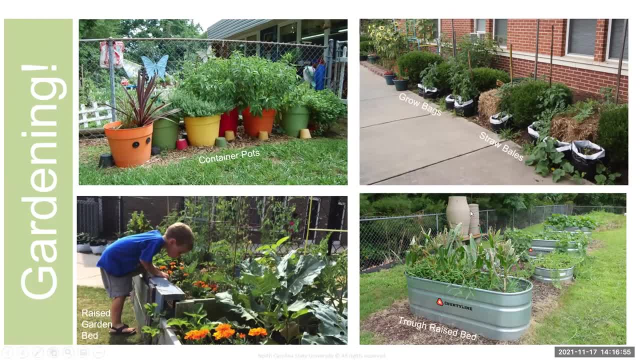 the fruit and vegetables in the garden beds, And then you can see back here they at this center or school. they have added in rain barrels to collect rain whenever it rains, or rain water whenever it rains outside as a way to water their plants in their garden beds. And then, of course, 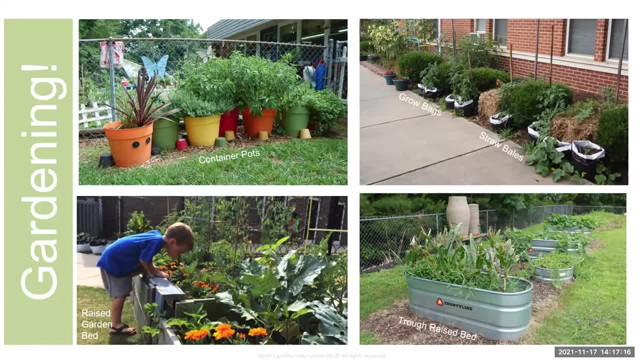 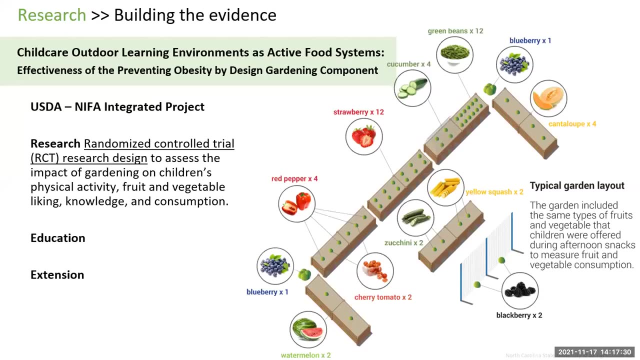 a raised garden bed or an in-ground garden bed is a great resource to use in educating children about different fruits and vegetables and just the whole gardening process, from beginning, middle and to end. So, before I touch on the guide that I'm going to mention, we did a, or we are actually still doing a research. 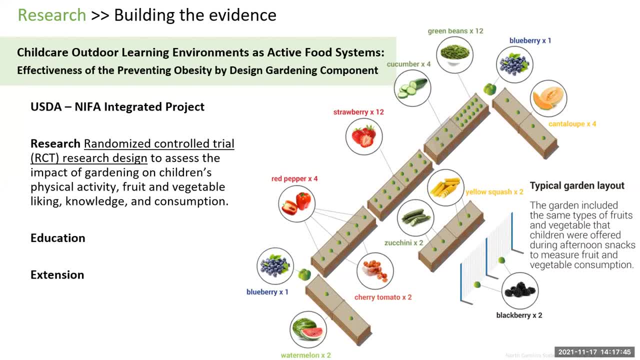 project with the USDA, which is a randomized control trial with 15 centers across Wake County here in North Carolina, And we wanted to assess the impact gardening has on children's physical activity, their knowledge and liking and then also their consumption. So at these 15 centers we put in raised bed gardens and we chose six vegetables and six fruits. 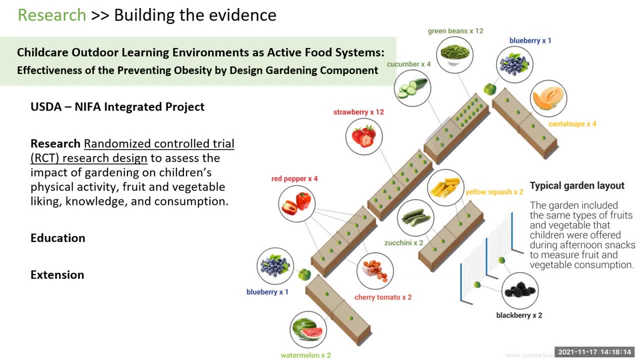 Only right now. here on this document, you can see five fruits. One of them that is missing is an apple, which they grow on an apple tree, so it can't be in a raised bed, But we chose these fruits and vegetables because they're easy to grow. 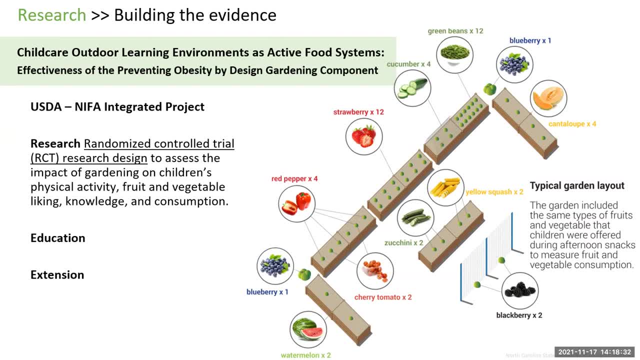 Especially with tomatoes they have now. I wouldn't say instant gratification for the kids where they can, instantly. it doesn't take as long to mature and to grow. They, over a few weeks, can start to see the the changes in that plant and at tours, when the fruit is ready to be harvested, they can. they can be grown in the garden. 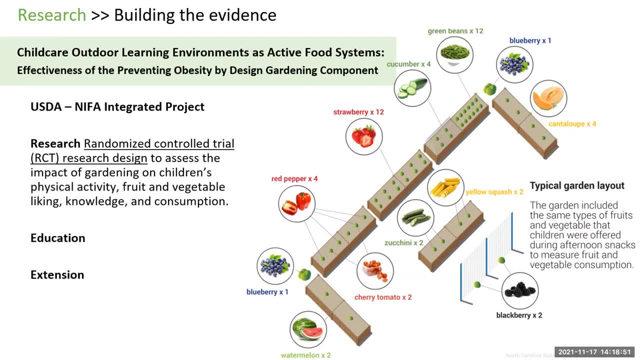 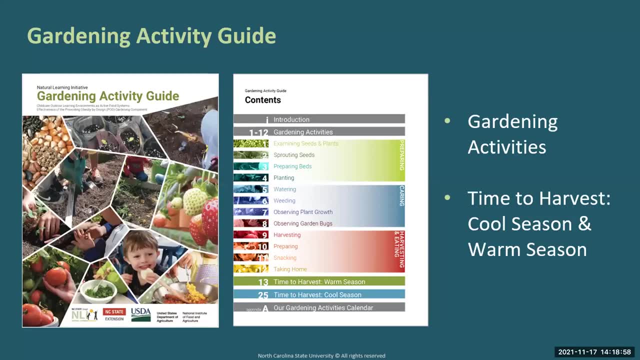 But we chose these fruits and vegetables because they're easy to grow, can try it right then and there. So, because of the research, we decided to create the Garden Activity Guide as a tool to help teachers, parents or any volunteers that are helping the center or 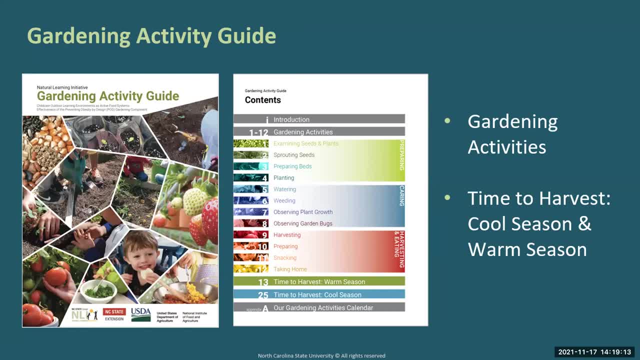 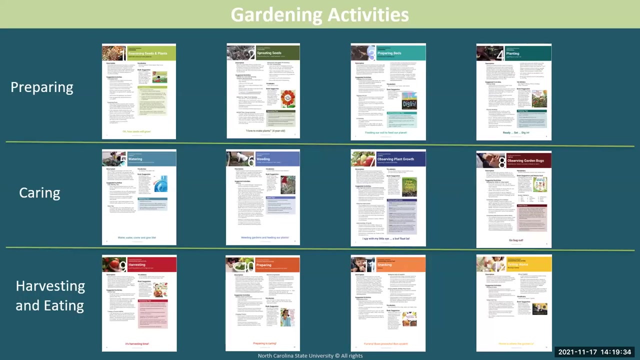 school, implement garden beds to educate children more about just the gardening process. So the Garden Activity Guide is broken into two sections, which is the Activity Section and then the Time to Harvest Section, which covers cool and warm season fruits and vegetables. So here you can see that the Gardening Activity Section is broken up into three phases. 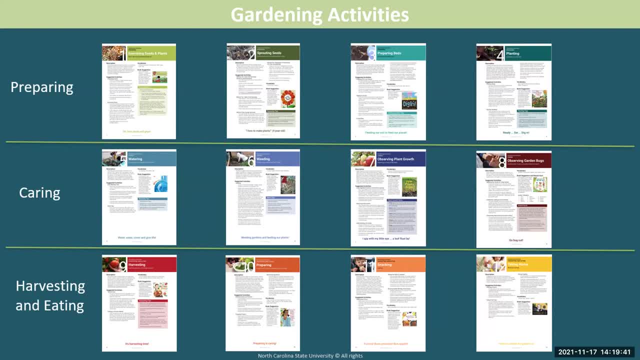 Preparing, Caring and Harvesting and Eating, And then within each phase there are four garden-related learning processes. So, for example, if you look at Preparing, in that phase it has examining seeds and plants, sprouting seeds, preparing beds and planting, And I'll go a little deeper in. 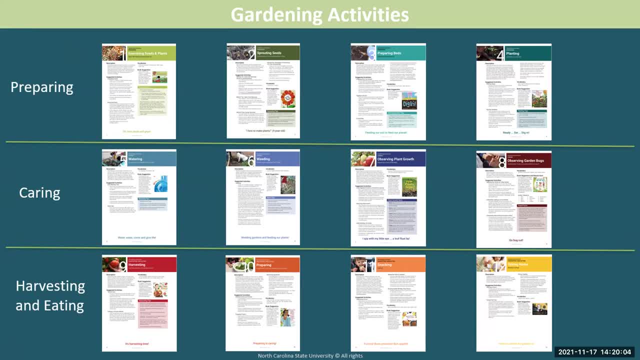 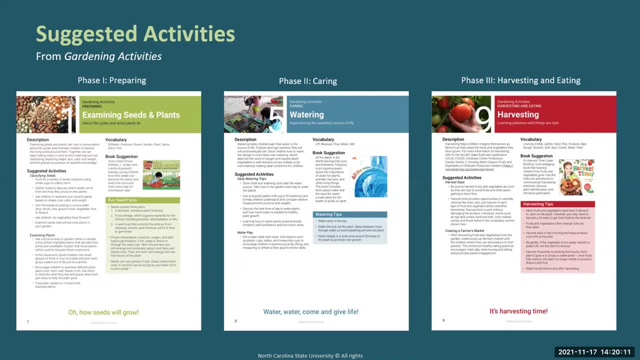 what each topic entails within the document. But this is just kind of more of a snapshot of a topic within each of the three phases And it kind of highlights just, for example, a description of that specific topic and then some more information tailored towards it. So we do recognize and, as I mentioned before, 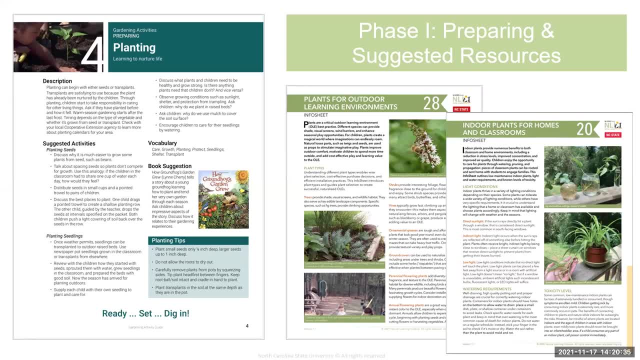 that this Garden Activity Guide is just a resource. It's not something that we are telling teachers, volunteers or parents that they have to use when working with children, Of course, as a professional or as a teacher or someone that specializes in gardening with. 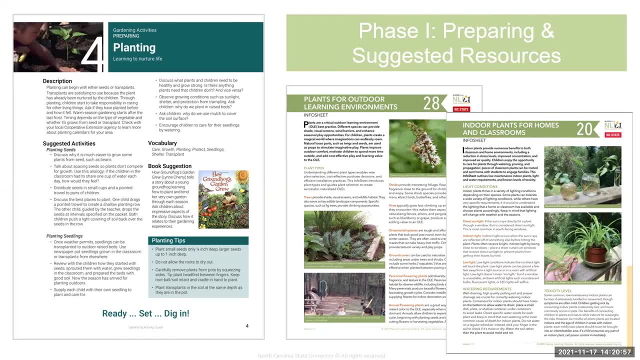 children. you are an expert in what you do And so you know, depending on the age group that you're working with or just the children's needs, what activities work best for them. But we also wanted to suggest going to our website and using some of the resources that we have online for free. 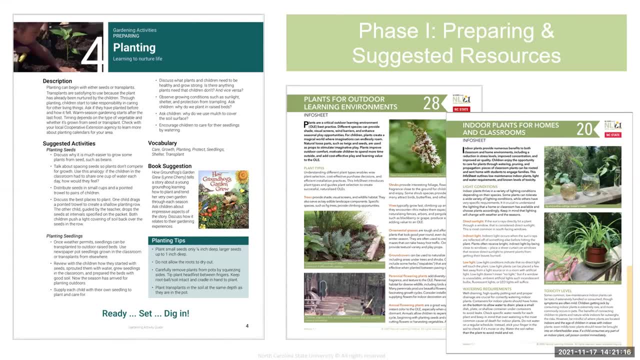 And so we have a lot of resources that go well with each of the different learning processes And so, for example, here you can see phase one, preparing. We're talking about planting, And we have two info sheets that talk about like, for example, plants for outdoor learning environments. 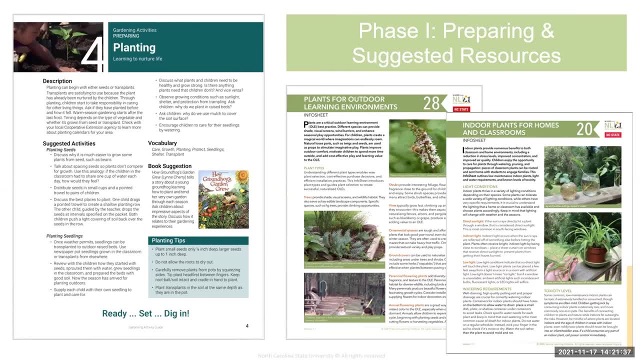 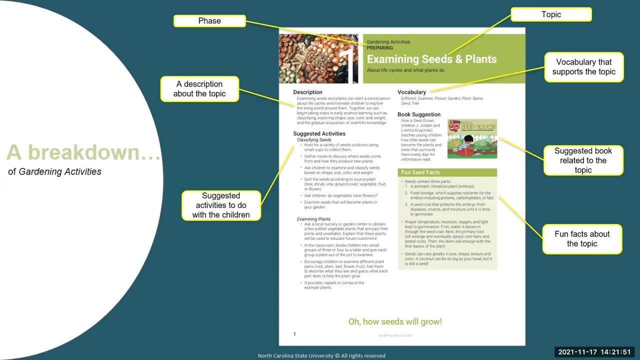 indoor plants for home and classroom that go or complement the actual learning processes associated with this particular phase. So just giving a little bit more breakdown of a garden activity section in a specific garden-related learning process. Here you can see that it shows which phase is in the actual topic of this document, a description of it. 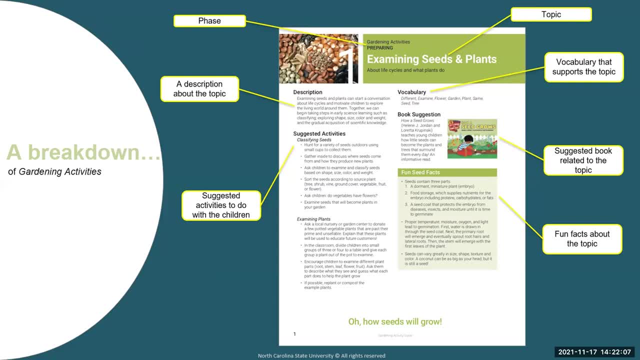 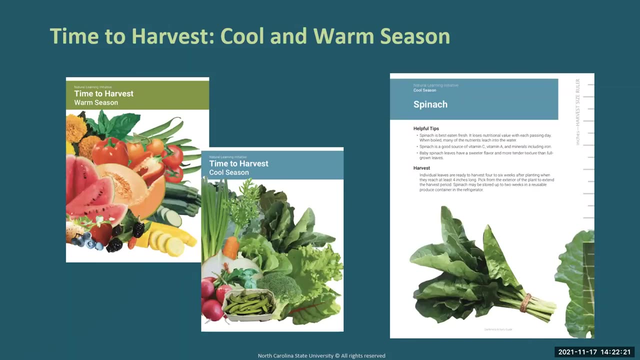 suggested activities that anyone can do with the children, suggested vocabulary books that are tied to this topic and then fun facts. So for the second half of the garden activity guide we have the cool and warm season section. So, as you can see, they're broken up into two parts: Cool and warm season. 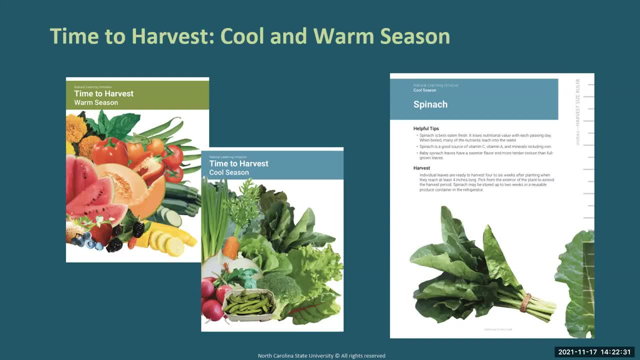 we each has about 12 different fruits and vegetables that are covered in each section, And then you know, for example, talking about spinach, it has helpful tips. And then harvesting um to help whoever's working with children or working with the garden. uh, determine when it's. 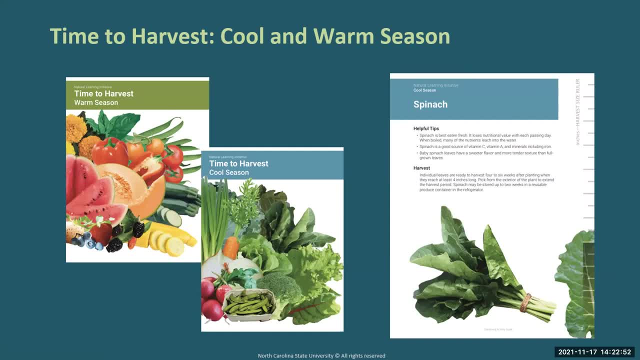 time to harvest that specific fruit or vegetable. if you look a little closer you can see- i'm going to move this right here- you can see there is a harvest size ruler. so this is just a tool that a teacher or whoever can use, especially if they're not familiar with gardening or they're not as 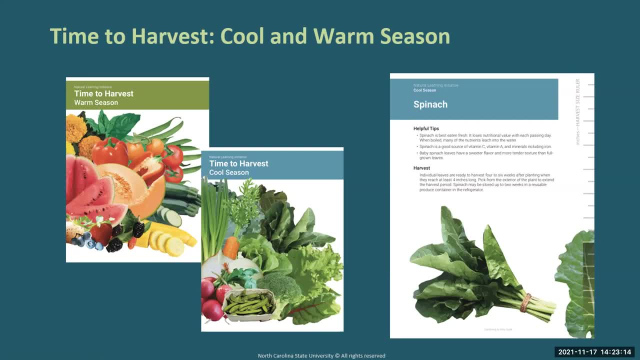 comfortable. they can use this when they are taking the children outdoors to determine whether it's time to harvest that fruit or vegetable based on their maturity. so they can take this document out outside, put it close towards, say, for instance, the spinach leaf and then, and by measuring that leaf, they can determine, especially with the information that's provided on this. 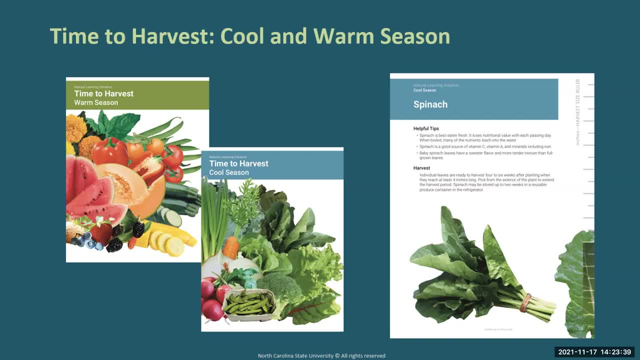 document whether that particular plant is mature enough to be harvested. now, we do recognize that this does not work for all fruits and vegetables, so say, for instance, watermelon or cantaloupe, which is determined by a different method, but we chose to add this just as a 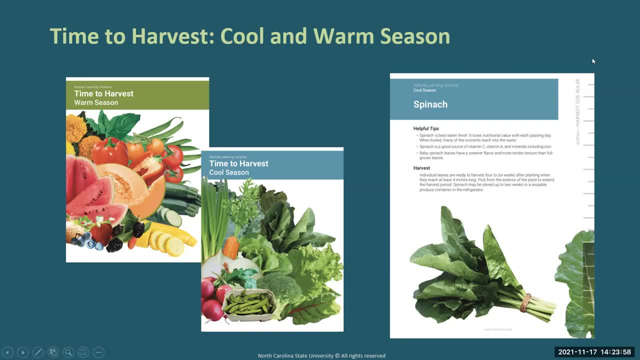 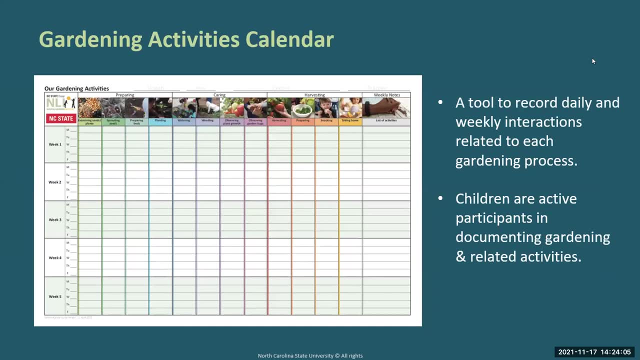 different helpful tool that can be used in gardening with children. so this is an addition that we added on, which is the calendar. so it's a monthly calendar, as you can see. it has five weeks, the days of the week. it also has the three phases of the garden activity guide and then the 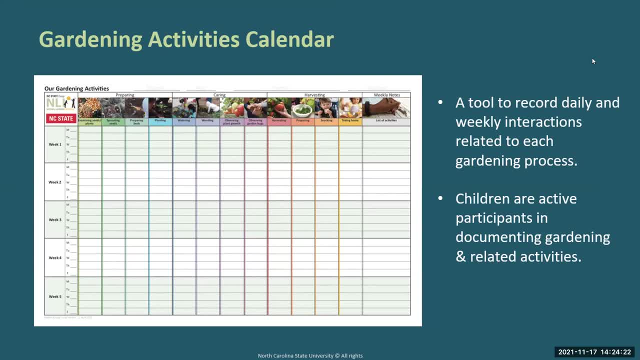 associating learning processes with them. so this is just a tool to record daily and weekly interaction with the garden. we highly encourage whoever is working with the children to document what they're doing so, either by writing notes and also by getting the kids involved while they're. working with the children, and then we do have more information on that as well. so that's what i'm going to be showing you, as i'm adding a table that looks like this or one that looks like this, and then i have another one. i'm going to be highlighting the slides that are mentioning for getting them as well. we have some. 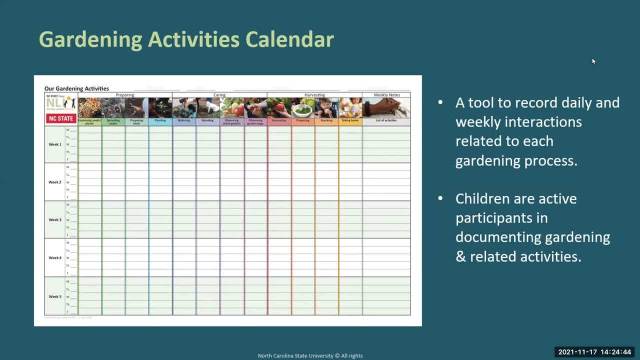 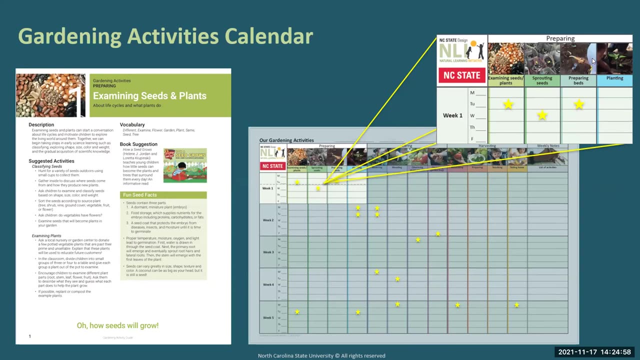 in the documentation of what's been done in the garden so the kids can be active participants by adding stickers to. so you can hear this. see this example: added stickers to the calendar are check marks or the teacher can just write dates to determine what was done on a pacific. 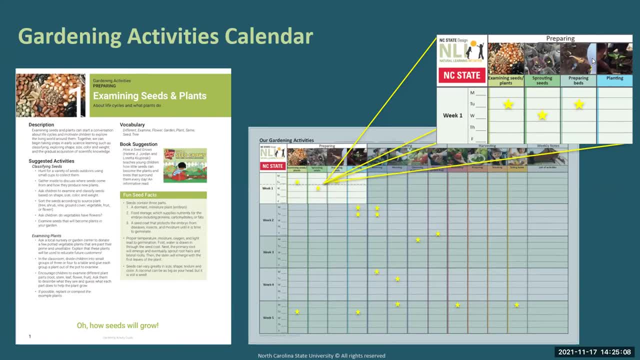 day or a week. um, we also highly encourage, maybe during small group time or during circle time, to just allow the kids be able to reflect on what they did that day, or maybe the day before the week before, to keep track of, um, the, the gardening experience, uh, throughout the 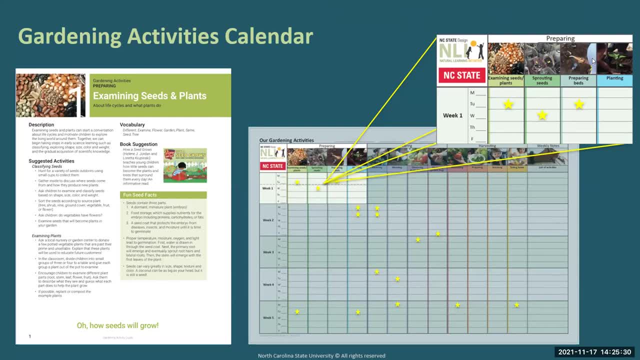 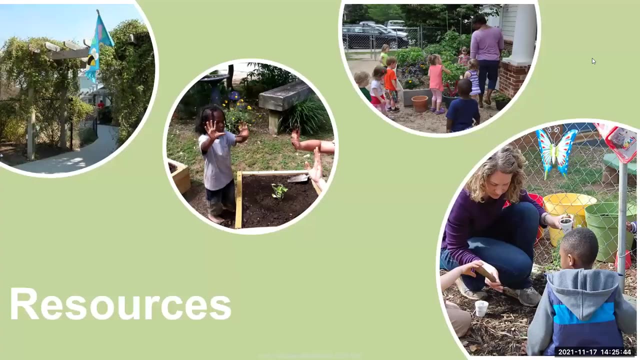 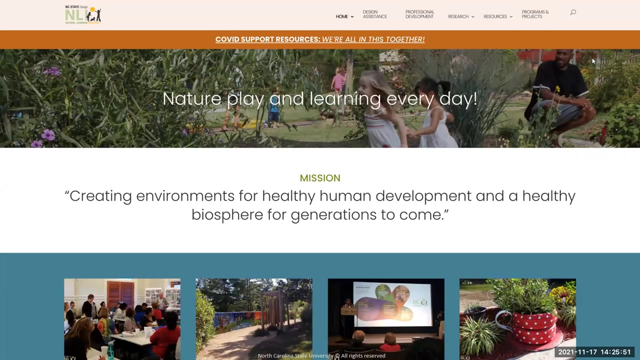 gardening season, um. so this is just a fun way to to get them engaged and interactive in the gardening and allow them to be independent thinkers and learner, learning learners during this process. so some resources that i want to touch on is, first, our website, which you can see a snapshot of it here, and we have our home page. we have the 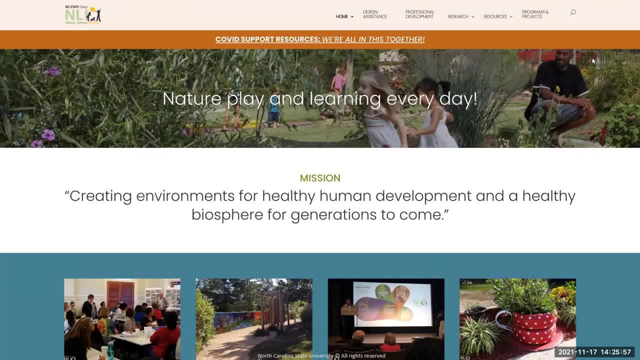 design assistance page where if you want assist assistants or someone you know who wants assistance in improving the outdoor learning environment or they have questions about garden care or other things like that, you can go to that page and fill out some information and we'd be happy to help them in any way that we can. we have a research page. we have the resource page also. 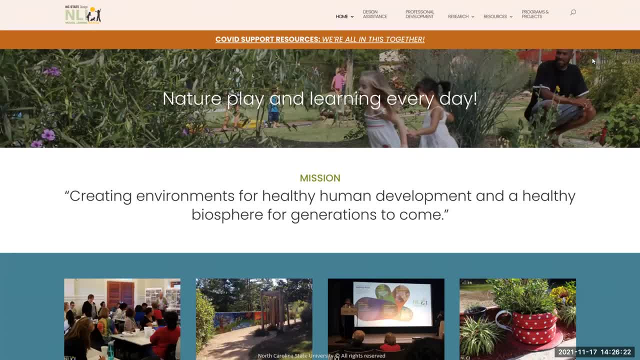 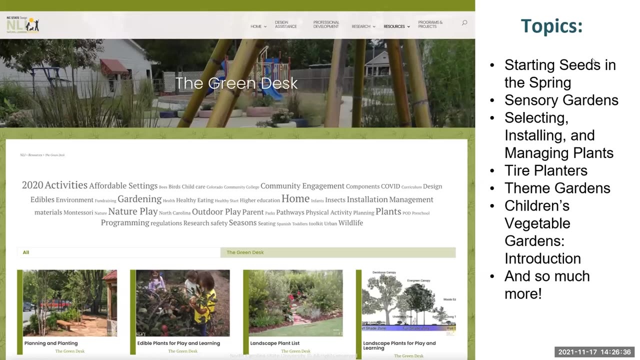 which i'm going to highlight some different things on that page, and then our programs and projects, which just showcases the many different projects that we've worked on throughout the years. and the green desk page started because over the years we get a lot of questions about gardening. 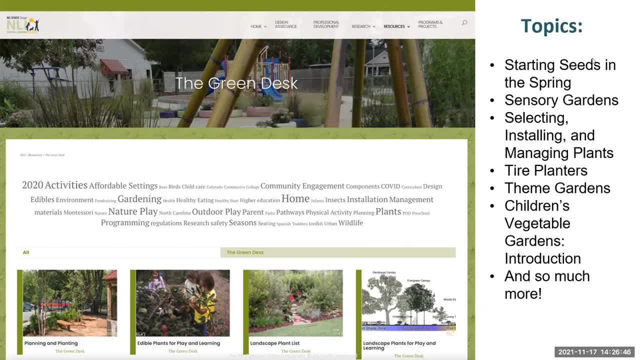 or the natural environment. so we wanted to have a page that hosted not only those questions but our responses to those questions, and so here you can see an example of some of the topics which some are starting: seeds in the spring, sensory gardens, themed gardens, tire planters. 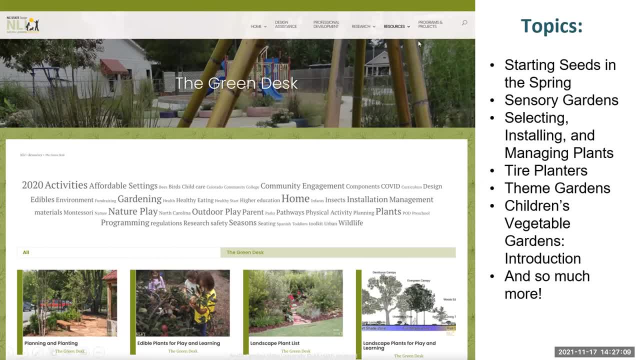 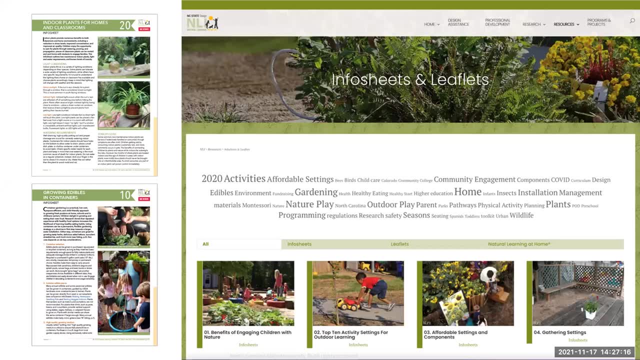 um, and then introduction to gardening with young children, to name a few. okay, so we have our info sheets and leaflet page, and so the info sheets, uh pages, are more in-depth information about gardening with children or about the natural environment, and so, for example, we here: 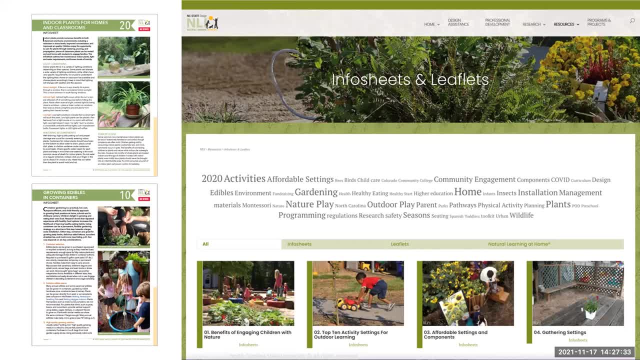 have information about indoor plants for home and classroom growing, edibles and containers. we also highlight the benefits of engaging children with the natural environment: um top 10 different activity, um activity settings and component components that can be implemented in the outdoor learning environment. we also highlight some of our 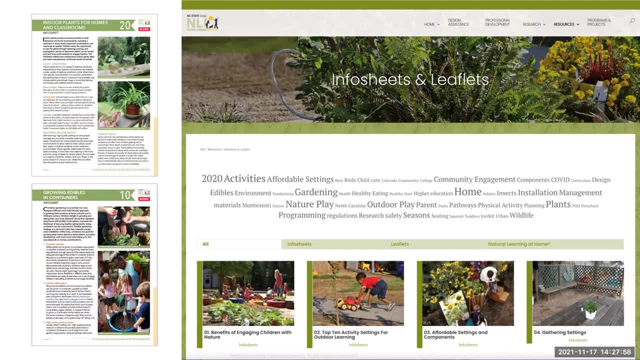 settings and components that we encourage centers or schools or zoos to implement, which one of them is um adding in uh vegetable gardening um, with the purpose of allowing children to be participants in those. oh, and back to leaflets. so leaflets are more like um activities that, uh, you could. 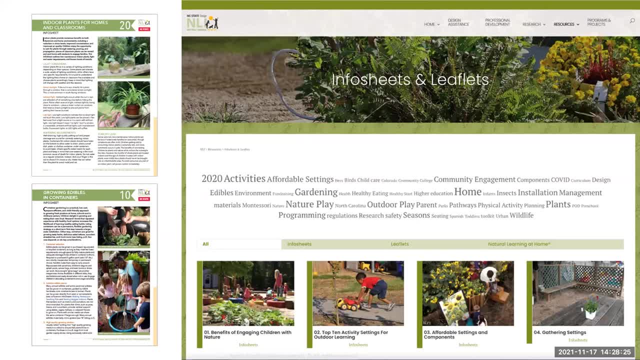 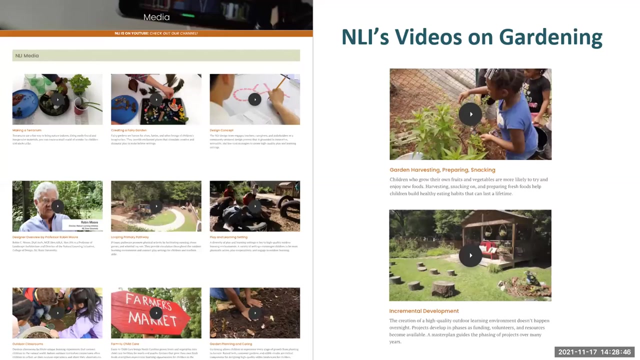 do with children on. so could be something um like um harvesting and eating sunflower seeds as an activity, with kids eating and sharing Um. it could also be creating trail mix um recipe, And so here we have our media page, which houses are the videos and just highlighting 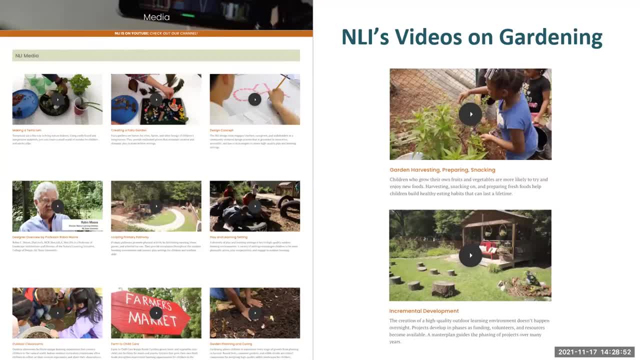 to. here we have videos on gardening. So this is harvesting and preparing and snacking with children and incremental development, Cause we all know, especially when you are working in an environment and you're trying to make it more naturalized, that it takes time. 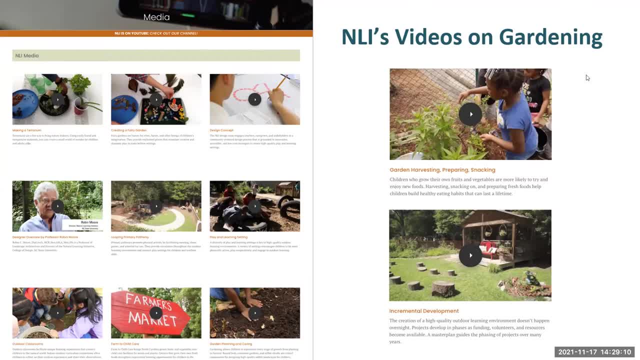 It's a process, Um, and so that's what incremental development uh video is talking about Um. we also have just different videos about how to create uh terrariums and fairy gardens, And then also what is design concept and kind of explaining what that means, um in a video. 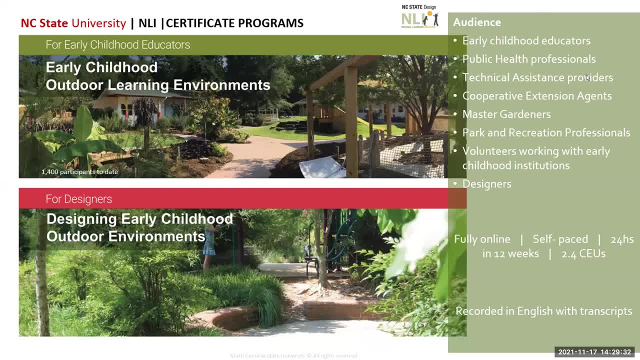 So here, as I had touched on before, is our certificate program. We have two. we have one that's geared to more gear, more towards um, early childhood, Um, and those audience are early childhood educators, public health professionals, master. 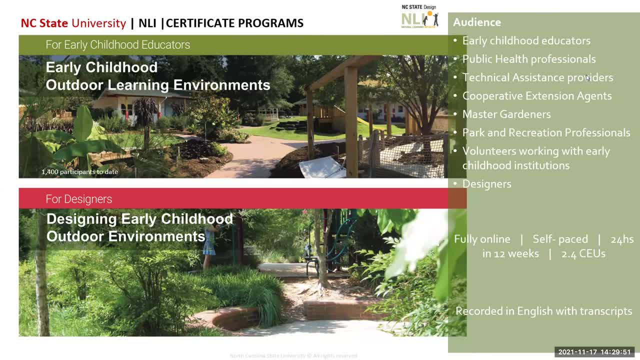 gardeners, parks and rec um volunteers. It could also just be parents who want to be more knowledgeable about um, learning how to implement or learning more about naturalized environment. We also have the Designing early childhood outdoor environments course, which is more for designers, people. 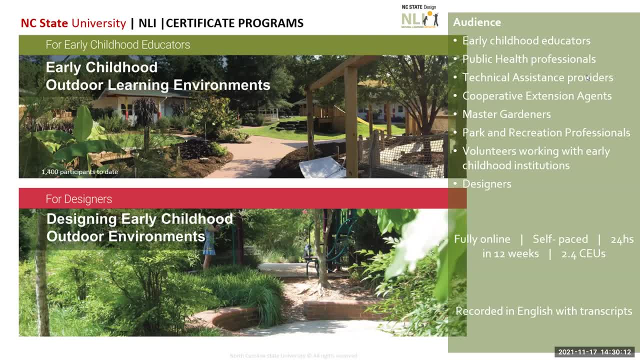 with who have a landscape designer background or landscape architecture, or who's able to, um, make scale designs. uh, could take that course. Now, these two courses are all online. Uh, they are 12 weeks self-paced um, and then at the end you can get up to 2.4 CEUs. 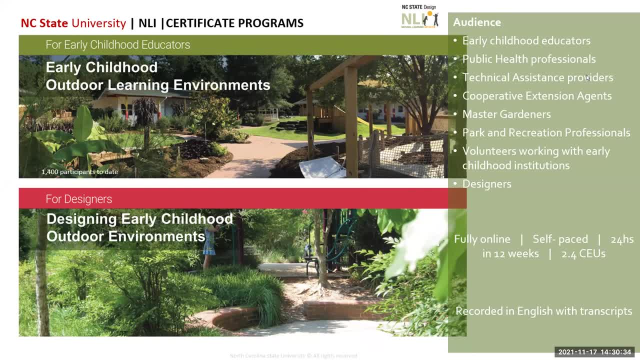 for taking this certificate course, And we typically have it three times a year: Um, we have one ongoing and then we have another one that's going to start February 14th 2022.. If you are interested in um taking that course, 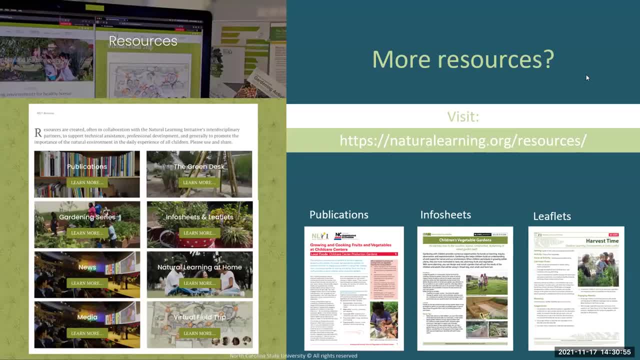 So if you want to learn more about our resources, I highly recommend that you go to our website. look at our resource page. Uh, I, we have some more things that I didn't even touch on. Okay, Oh, there's one there. 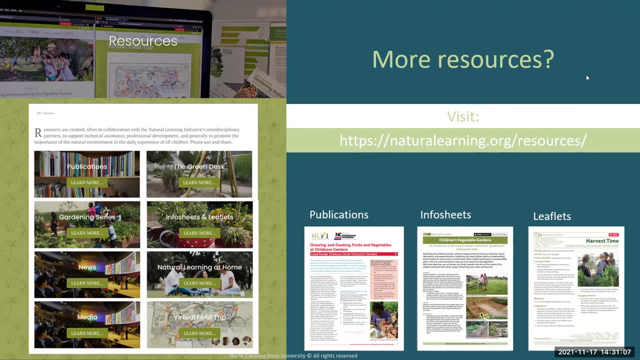 Oh, there's one there. like our publications, our gardening series that we did with Cooperative Extension, We have our Natural Learning at Home, which is our parent engagement series. We have a virtual field trip which I strongly encourage everyone on here to go and check out. 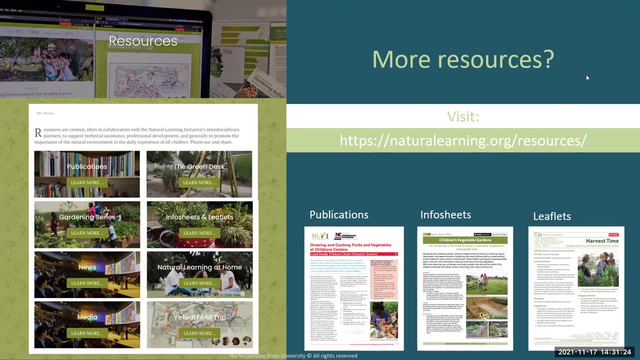 which is just a field trip around a childcare center, highlighting different naturalized activity settings and components. And then there's an interview by two directors and also the director of Natural Learning Initiative. Even if it doesn't, maybe you're working with older children. 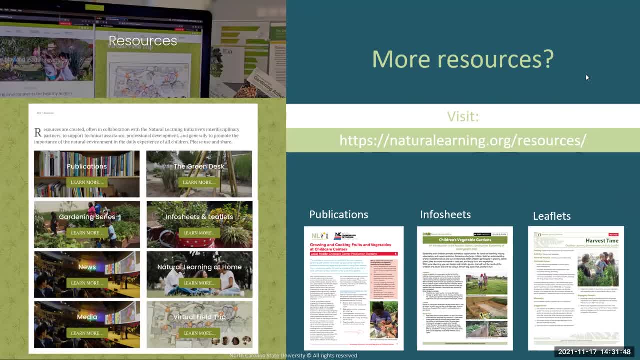 I think it's still beneficial to come and check out what we have, check out the virtual field trip, even though that's geared towards child development centers. There's a wealth of information that is shared, that is not tied towards just that age group, that it's beneficial to have. 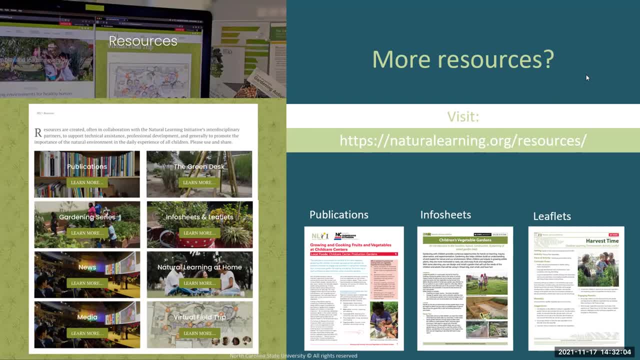 It's beneficial to anyone who wants to educate children about gardening, or you wanna learn about creating a more naturalized environment, especially now, with everything that we've been through, we all now can recognize being outdoors is beneficial for our health and also for the education. 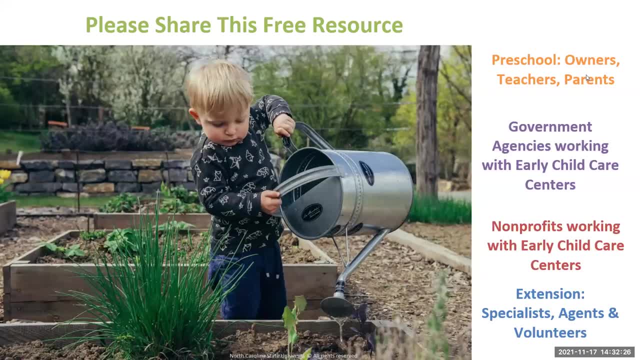 of our young children. So please, like I said, go to our website, check out our resources. They're geared towards people in early childhood field, government agencies, nonprofits who work with early childhood professionals, and then extension agents or individuals like yourself. 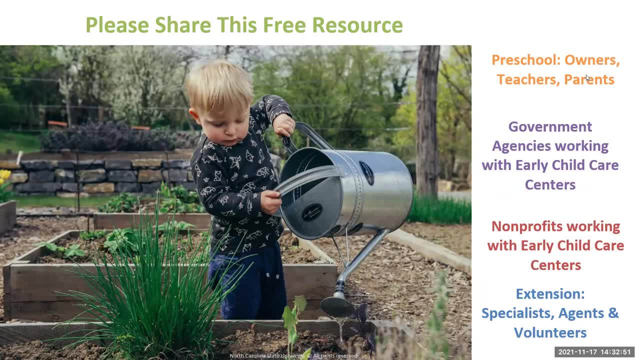 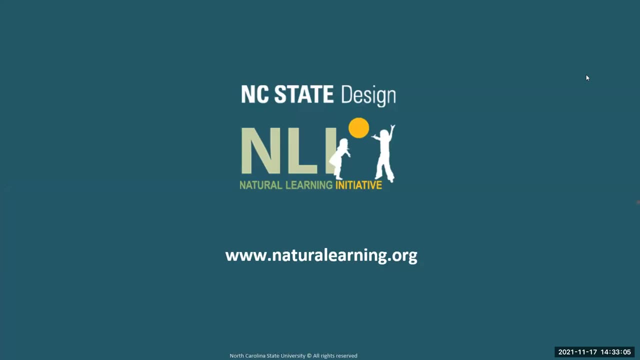 who are master gardeners and do this as your job or a hobby, or as a part-time job. I highly recommend you go and check out our website. Thank you so much for allowing me to speak about what we do here at the National Learning Initiative. 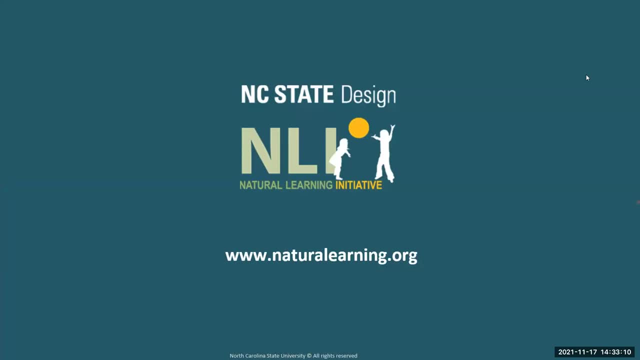 and one of our big resources- that we just pushed out the Garden Activity Guide. I will mention before I end that we just completed the Garden Activity Guide on semi-arid areas And so hopefully that should be on our website soon, but you can go to our website and see the initial one. 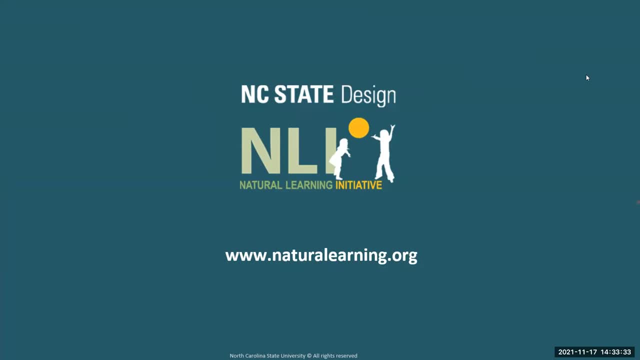 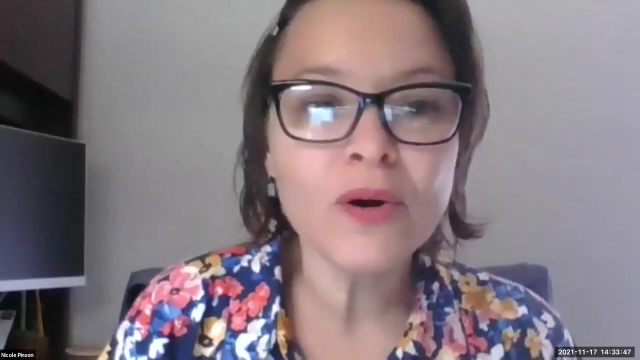 one that we did in connection to our USDA project. But again, thank you so much for allowing me to be here to speak and let me know if you have any questions. Thank you, Bria. So we're gonna hold your questions until after Carolyn's presentation. 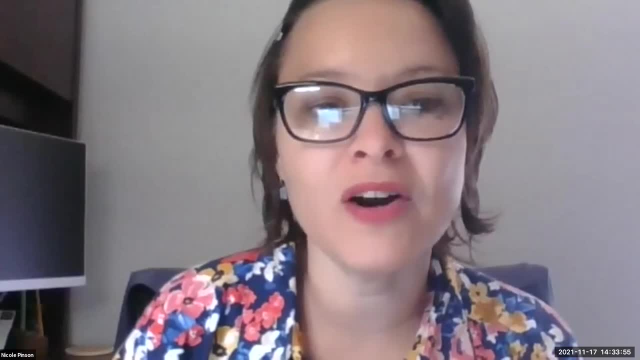 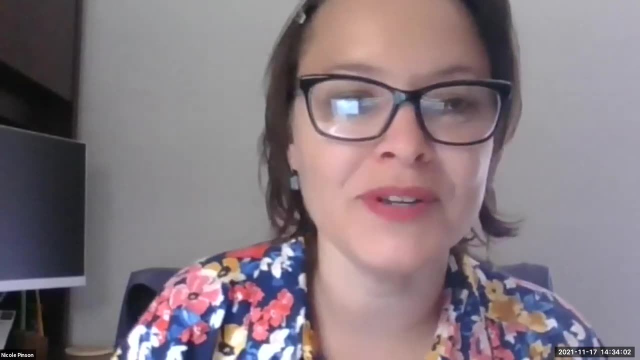 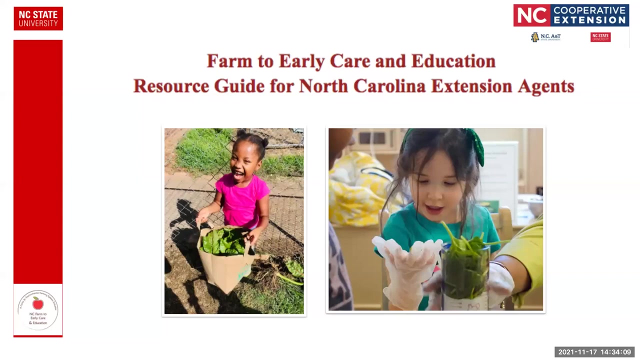 and then we'll go over everyone's questions and comments. We have a lot of good comments already coming in the chat box. All right, So we're gonna hang tight and Carolyn's gonna do the second half of the presentation today. Can you see, okay? 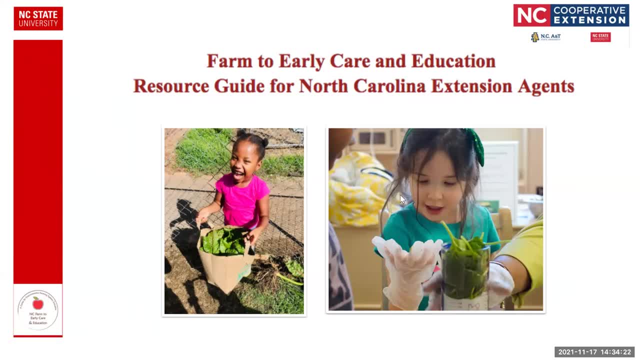 Yes, you're good, Okay, awesome, Yay, Cool. Hey everyone, My name is Caroline Hundley and I'm here to talk to you about a resource that is in development, but it's almost ready, So I'm really excited about this. 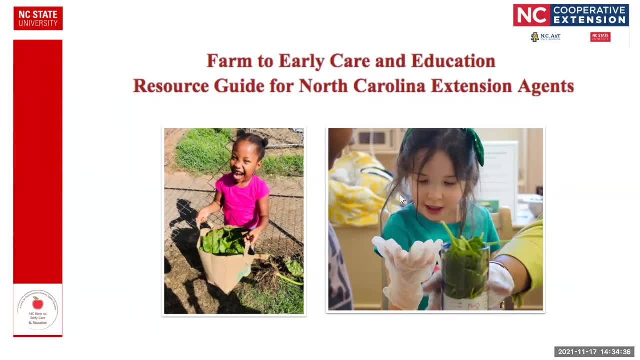 especially after hearing about Bria's awesome work and all of the resources that she has. those will actually be nested within this document so agents can refer to it. But I'm gonna talk a little bit more about farms, early care and education more generally. 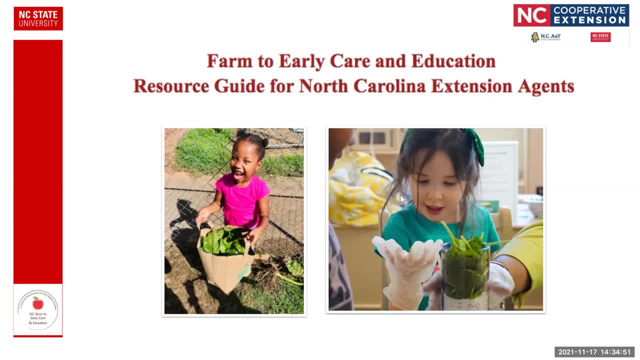 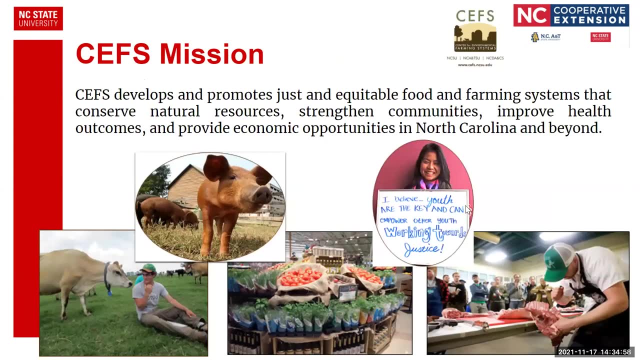 and then about this guide that North Carolina is developing, So I'm excited to share this with you. So first, just a little bit more about CESS. So the Center for Environmental Farming Systems- the systems that I work at- is a three-way partnership. 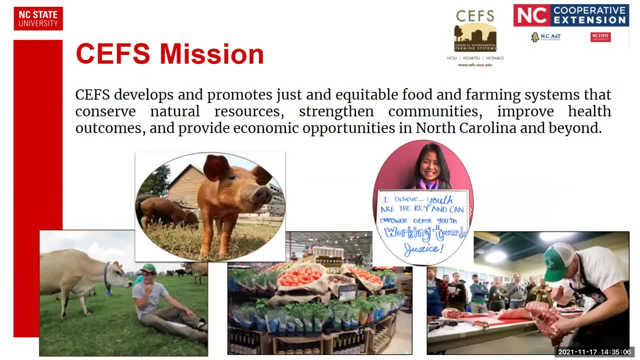 between North Carolina State, NC A&T and NC Department of Ag, And our mission is to promote just an equitable food and farming systems that conserve natural resources, strengthen communities and improve health outcomes, as well as providing economic opportunities for North Carolina, And so our vision is all about vibrant farms. 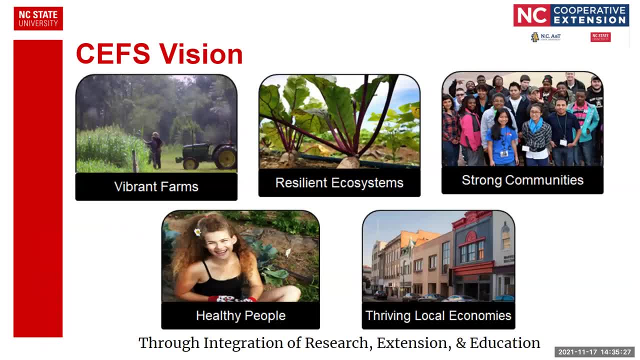 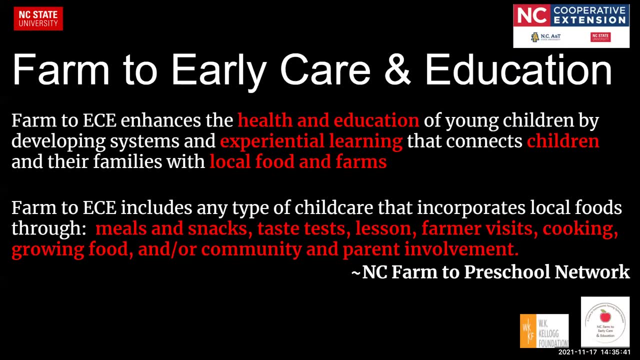 healthy people, resilient ecosystems, strong communities, thriving economies- all of that. And we do that through extension, And so you can kind of see how farm to early care and education can fit into that mission, as well as how Bria talked about all of the gardening. 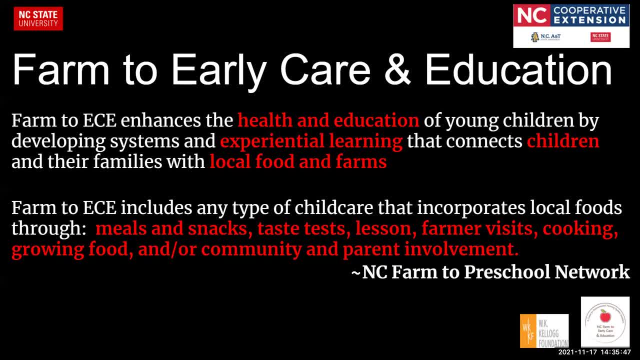 and kids really learning and understanding where their food comes from. the importance of all of that- Farm to early care and education, or farm to ECE- is all about the health and education of young children, experiential learning, connecting with their families. 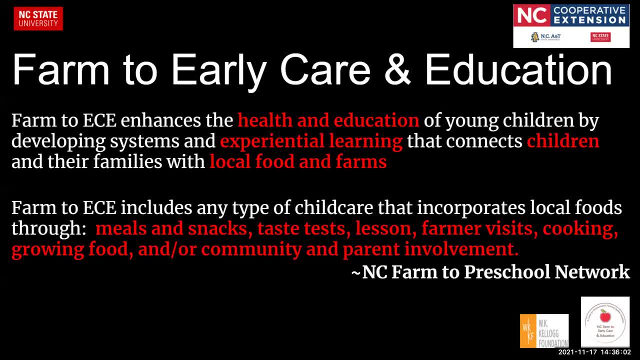 connecting with families and connecting them to local foods and farms, So it's anything that kind of incorporates local foods through meals and snacks. So doing that local food procurement and purchasing from centers and taste tests to really get children to try new foods and appreciate new foods. 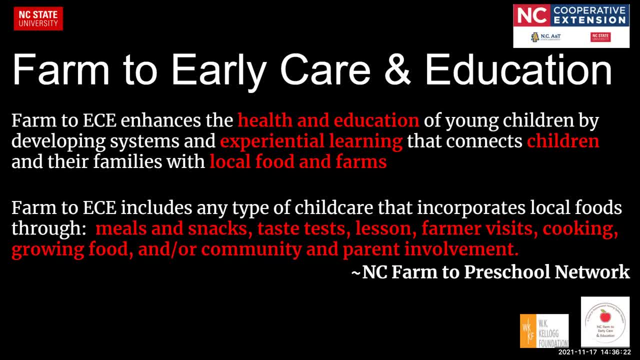 connecting to the curriculum through lessons, farmer visits actually into the classroom or having children go out to do farm visits, cooking and growing food, and that community and parent involvement. So farm to early care and education. I mean we really think about anything that helps children. 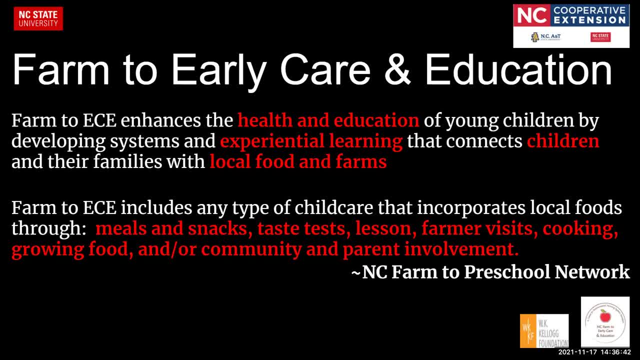 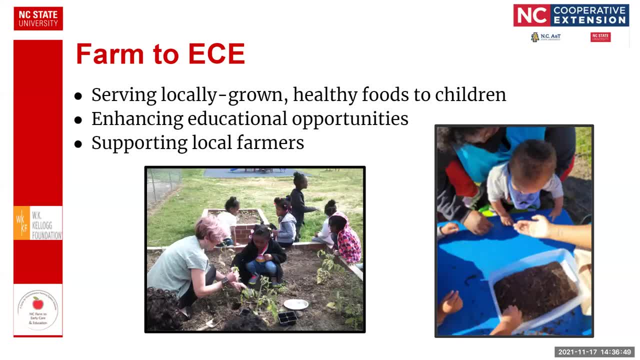 understand, know and love local food and where their food comes from, and getting So that locally grown, healthy foods to children, enhancing their educational opportunities. We like to make sure that teachers understand that this is not something necessarily extra that they have to do in their classroom, but it's something 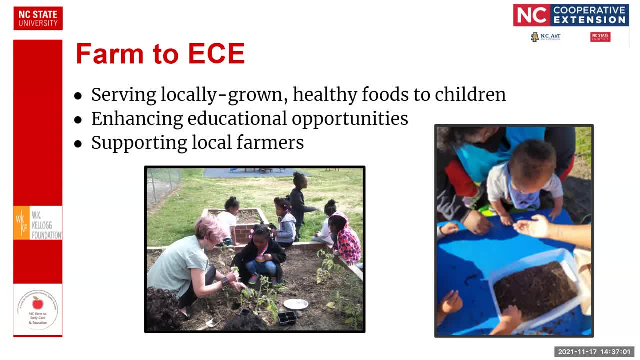 that they can do in their classroom, but it's something that they can do in their classroom, but it's something that they can do in their classroom, So that it's something that really fits into the curriculum, so that it's something that children become familiar with on a daily basis. 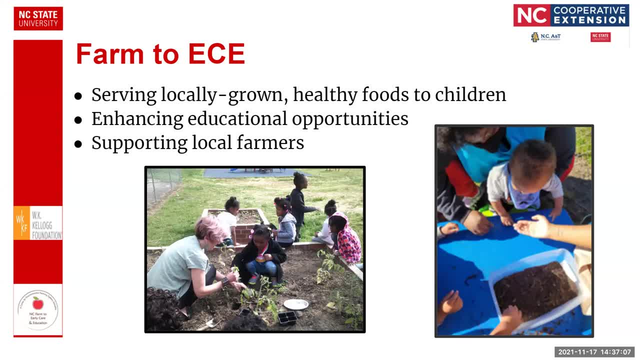 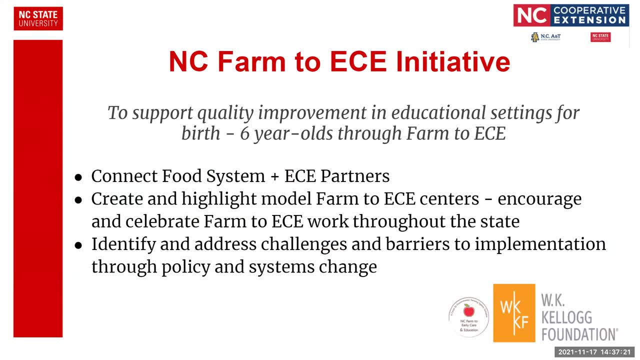 Like they just know that. you know they go out into those gardens and learn and play and that's just a part of their classroom culture, their school culture. And then, of course, we love that it supports local farms. So our initiative, CES, has a lot of local food initiatives. 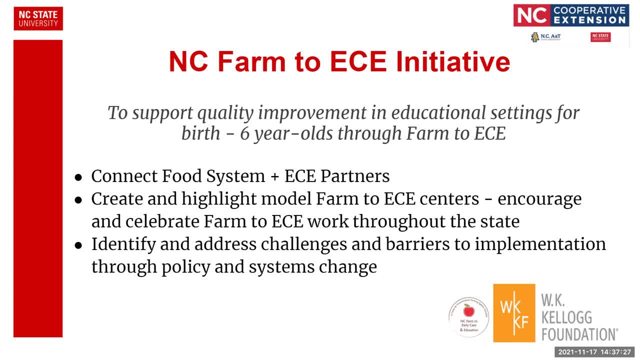 where we like to get local foods into institutions, And so farm to ECE is just like that. So we really want to support the quality improvement in educational settings. So for farm to ECE that's birth to six, So it's any kind of preschool classroom, infant toddler classroom. 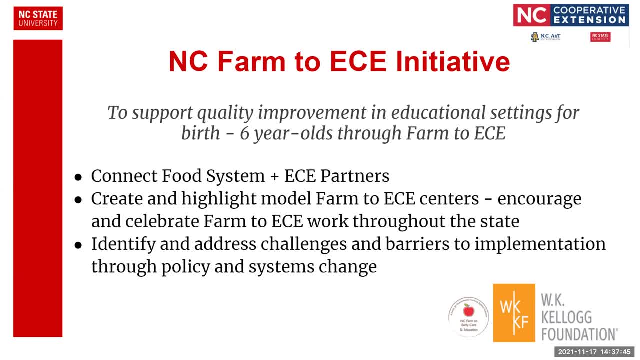 headstart, early headstart- any of those educational environments where young children are. So we do this by connecting food system and early childhood partners. So locally, that looks like connecting extension with the childcare community, which is what the guide is all about. 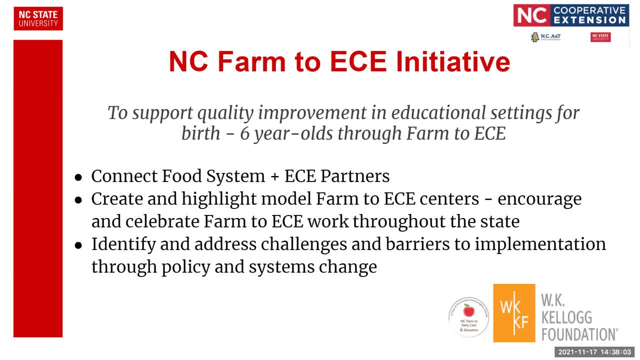 And then we want to also, with our initiative, really create new model farm to ECE centers as well as highlight the folks that have been doing this for many, many moons. Some of those pictures we'll have on this presentation as well. And then we want to, of course, 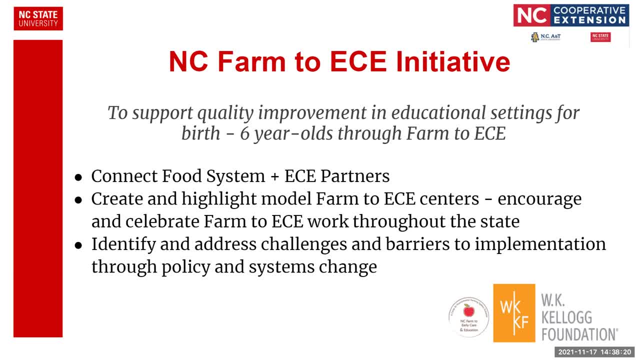 encourage more farm to ECE work throughout the state, And we do that by identifying and addressing the challenges and barriers that folks are experimenting now. So you know, why aren't they building those gardens? Why aren't they building those gardens? Like what's stopping them? 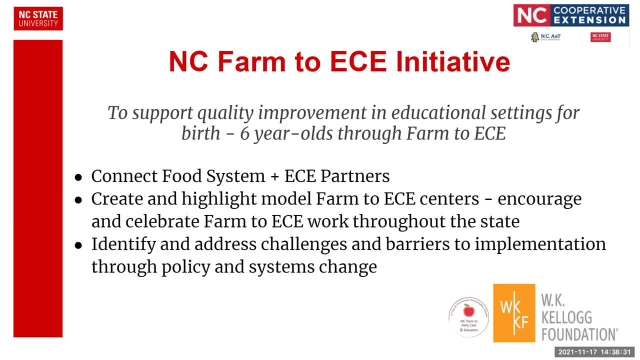 Like what are kind of systemic reasons that they're not building them And how can we kind of help change that on a systemic level? So, as we said, we are trying to connect those food system and ECE partners but traditionally extension in the childcare community from surveys that we've done. 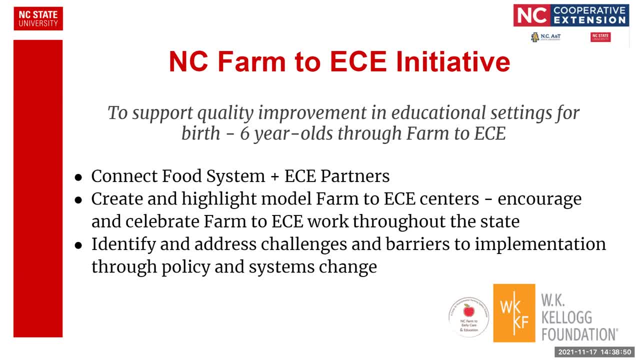 with our extension community. that is not something that is just the natural kind of go-to partnership. So a lot of times they'll serve on each other's boards and that kind of thing. But generally- and this is with a lot of partners that we work with- they normally go to the K-12 arena to work. 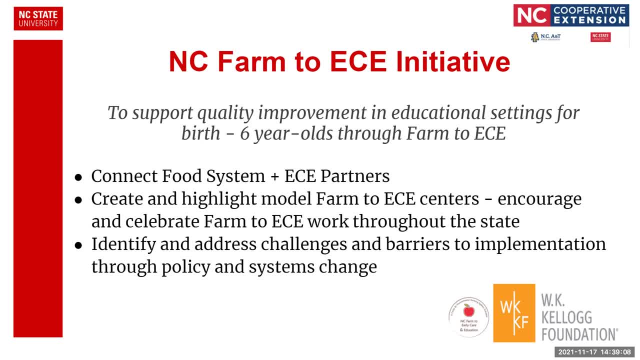 with children and families, But that early childhood is not something that they necessarily have thought of as a likely partner or somebody or people that can benefit from this work, But young children and their families. this is when you know their taste buds are developing. 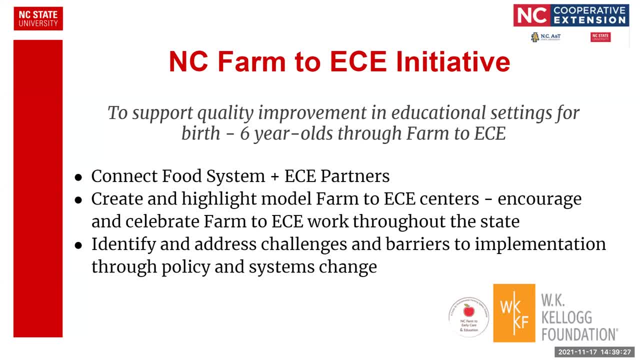 They're really getting might be their first opportunity- opportunity to taste this new food. It's just such a wonderful age to get started in this work, And so we really are so excited to work with an extension to kind of promote early childhood as a really exciting partner. 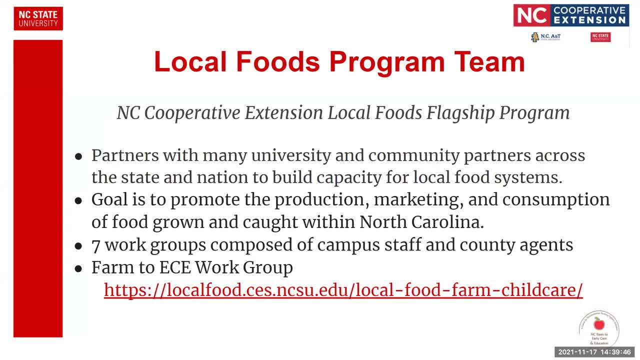 So I also want to touch on our local food program team. So this is our Cooperative Extension Local Food Flagship Program and the goal is to promote local food And we have seven different work groups that all have this mission of promoting the production, marketing and consumption. 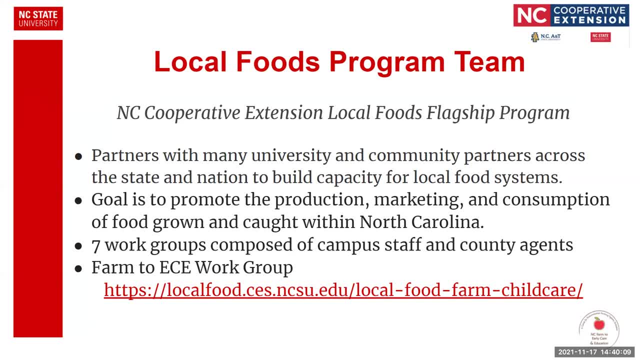 of local food in North Carolina. So the Farm to Early Care and Education Work Group is one of these seven, And so our work group. this is a link. Let's see. I know you've been putting stuff in the chat. I was wondering if you would add this general website. 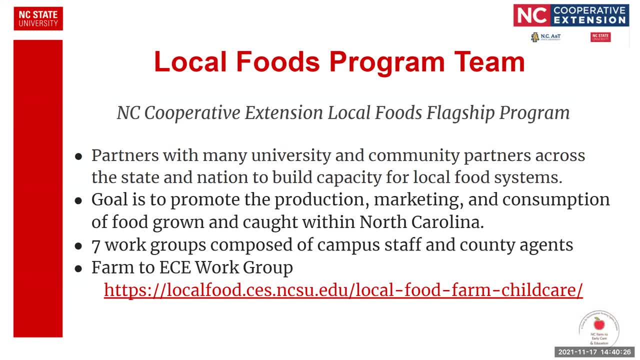 into the chat, but this is more on Farm to Early Care And so we have a lot of resources that are for childcare more generally. So we call it Farm to ECE, You can call it Farm to Childcare. You might hear Farm to Preschool. 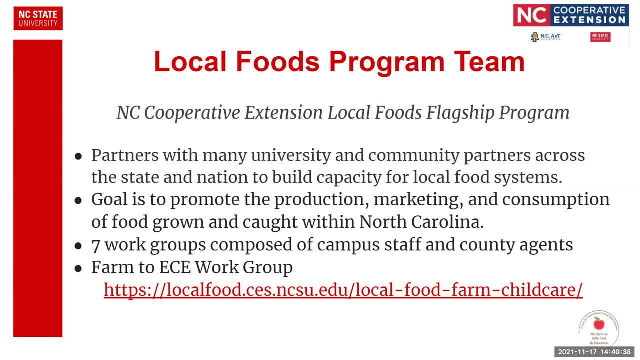 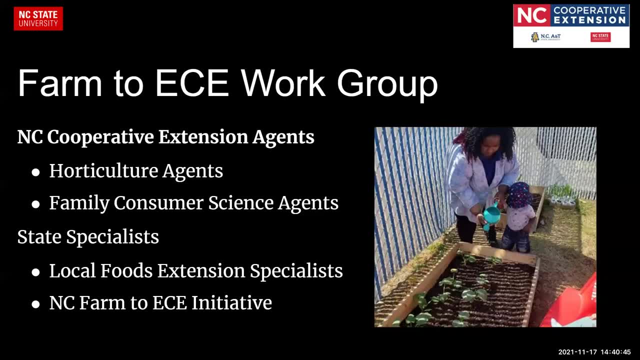 But that has a lot of Farm to Childcare resources more generally that the work group has compiled, And this is who's in the work group. And then I'm going to touch on the new guide that we've created that we're really excited about. 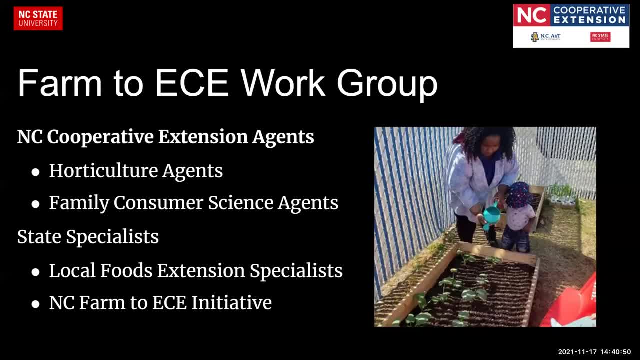 So typically all of our local food program team work groups are campus and county driven. So we have two co-chairs, One from campus and then one that's a county agent, And then we like to make sure that there's both of those agents and the specialists involved. 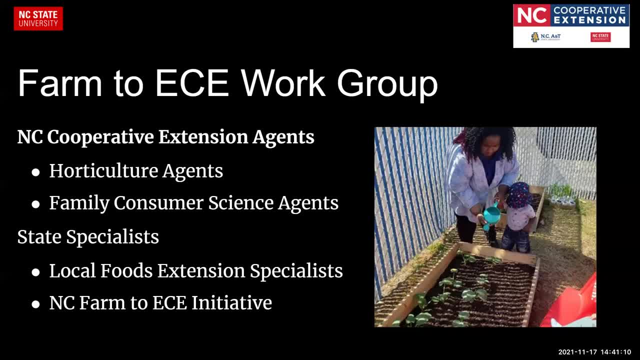 So we have horticulture agents, family consumer science agents mainly, and then we have state specialists like Lucy here and folks that provide support to family consumer science agents, And then myself and our initiatives training coordinator are all on the work group, So we work together to support agents. 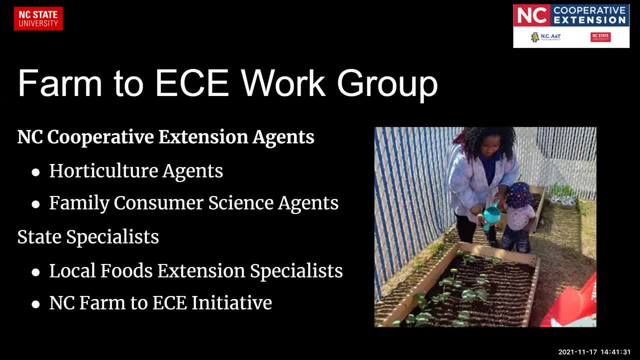 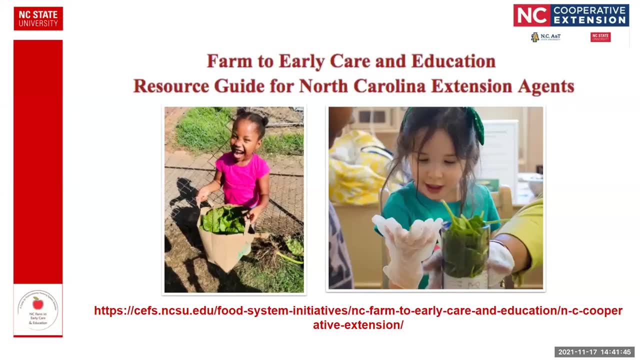 and how they can promote local food to the ECE community. That's our mission. And so now for the resource guide. So here's our link to where the resource guide will be. So this is actually our initiative's website, And we have tons of so many resources. 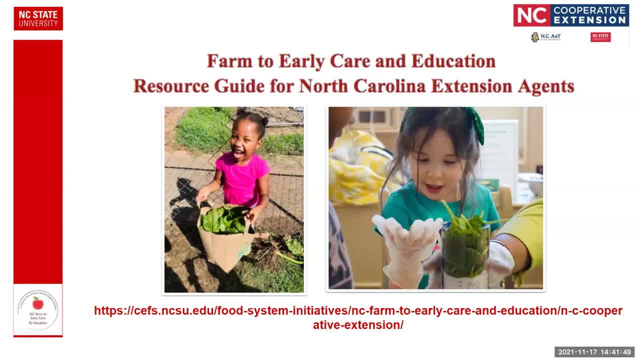 for both agents- ECE providers, teachers, parents- Everything that we've done through the six years of our initiative. So we have a lot of resources on this web page And we have some success stories of extension agents that are doing farm to ECE. 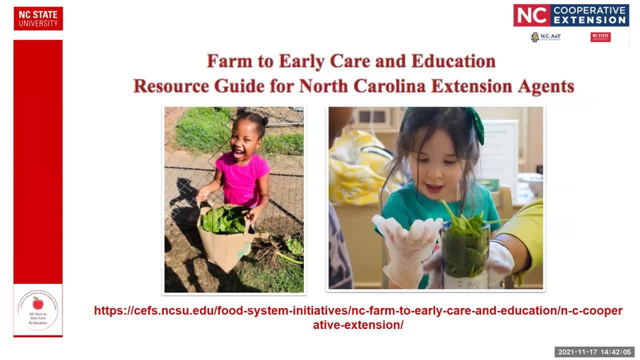 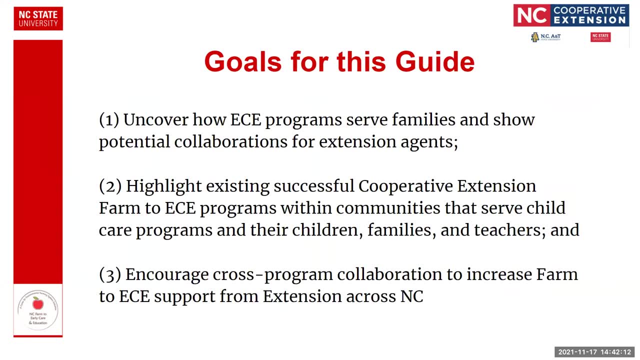 So definitely check that out, But that's where the resource guide will live, as well as the link that Lucy is sharing, And the goals for this guide is to really essentially, if an extension agent wants to crack into the ECE community, that might be just a brand new place. 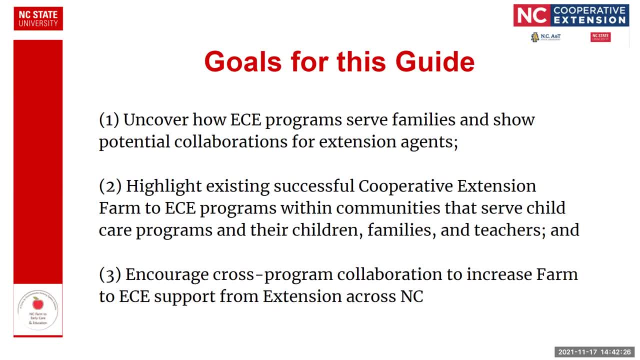 Right. So how can we make it easy? It's great. It's great. It's a great way for extension agents to do work with young children, their families, teachers, et cetera. So we want to uncover how they can serve families. 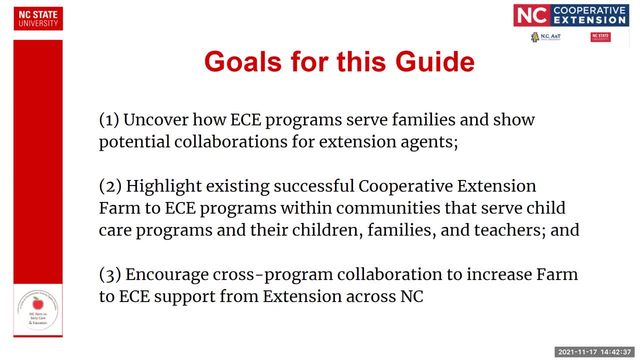 and show those potential collaborations. So just waving our hand and saying, hey guys, remember the ECE community. This is such a great place for you to do your programming and to really branch out to new populations. Highlight existing successful cooperative extension programs. 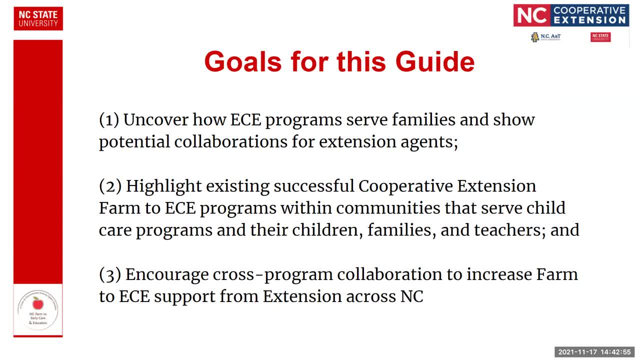 We have a lot of success stories nestled in our guide that are really fun and exciting. and then we've also found that this work in particular encourages cross-program collaboration. so we've had family consumer science agents work with horticulture agents, local food agents, ag agents, you know for that farmer connection. so we definitely want to 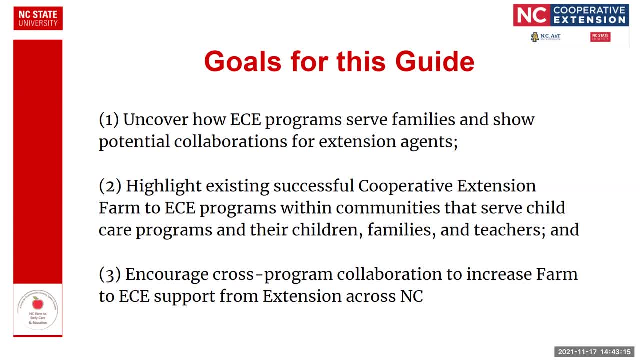 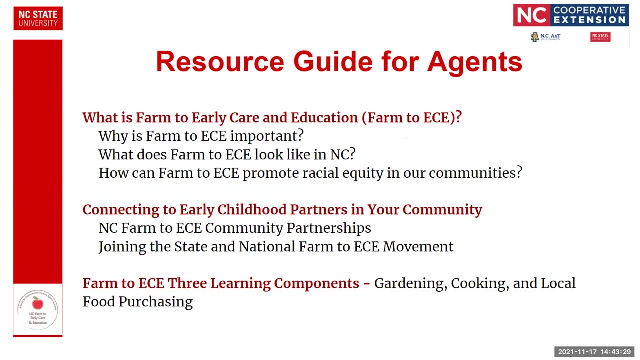 highlight that and provide ideas for agents through this guide. so this is just a little bit of an outline of the resource guides. so we start with what is FarmTEE? a lot of folks have heard of farm to school, um, so we like to say: you know that it's farm to school, but for the itty-bitties. 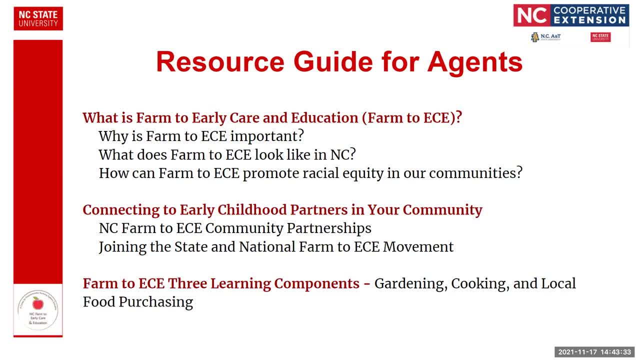 right and we talk about why it's important. what does it look like in north carolina? there's a lot of institutions that play in north carolina, which is really helpful when local folks are trying to uh kind of partner with child care centers in their area. they're trying to you. 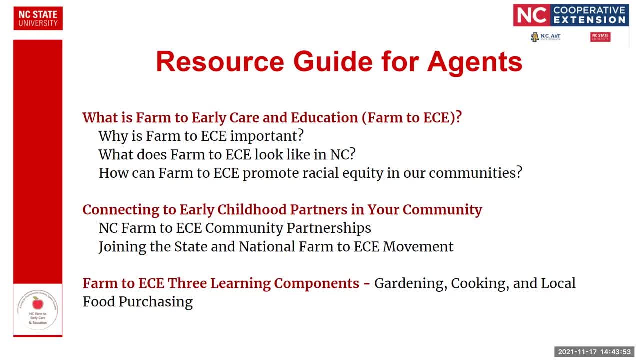 know there's institutions in North Carolina, Southern California. you know you're trying to. you know there's institutions in North Carolina, Northern Carolina, you know. you know they're trying to, where they can just go and say, hey, link me up with this type of classroom. 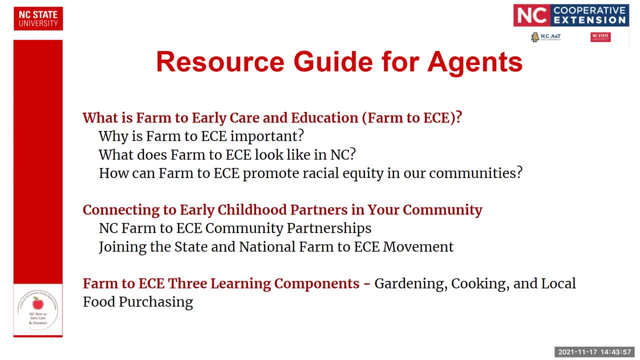 this type of program, So that's really helpful in North Carolina. So we do outline some North Carolina specific resources in here. We talk about how Farm to Ease can promote racial equity in our community to ensure that everyone, and especially the folks that most need it. 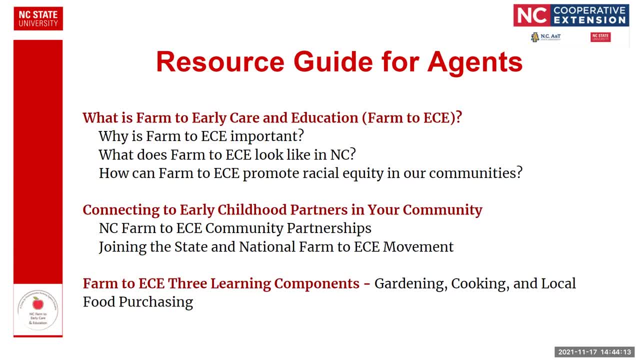 are receiving this education, And also just that our programming is equitable and reaches all folks Connecting to early childhood partners in your community. So I talked a little bit about this. but we also have state and national movements that folks can connect to, So a lot of agents don't know. 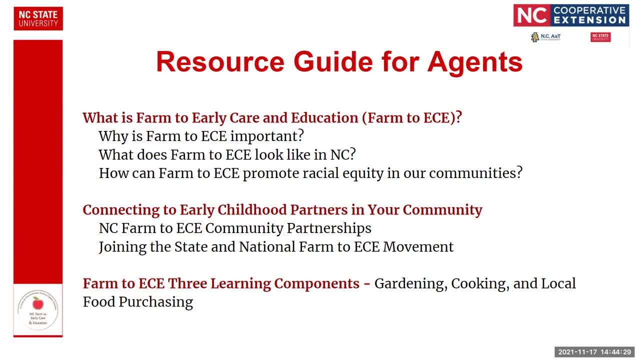 about the National Farm to School Network, or we have a statewide North Carolina Farm to Preschool Network that they can join, And so a little bit about that is gonna be in there, And then we go into a little bit more detail about what this programming actually looks like. 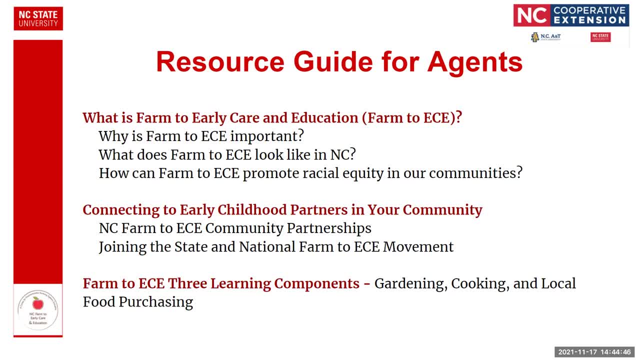 So we have three learning components that we've organized it into. We have gardening, cooking and local food purchasing, And so for the purpose of this presentation, I now have about five minutes left. I think I wanted to just go into a little bit more depth. 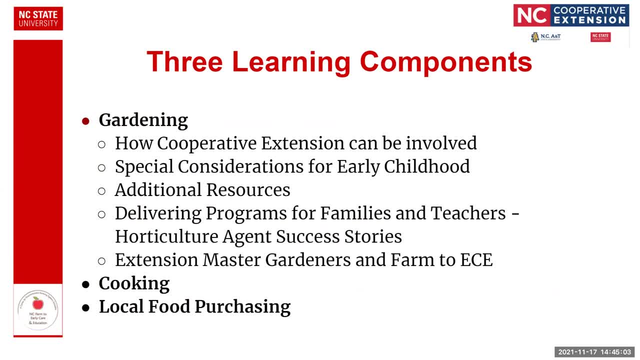 about the gardening section and a couple of teasers for y'all. And then, of course, the cooking and the local food purchasing sections near this gardening section. So we start with how Extension can be involved in special considerations for early childhood. Well, we also do that in the cooking and local food section. 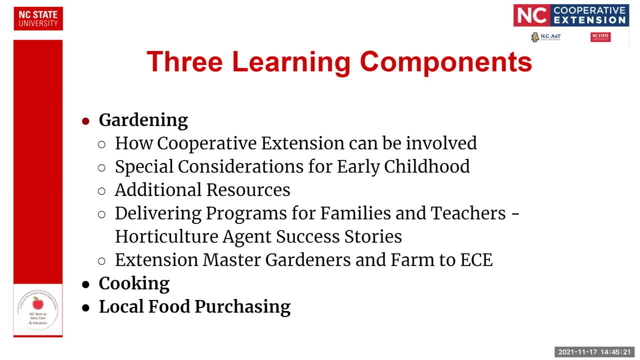 So you can kind of get an idea of what the guide is going to look like more generally as well. So that's how we start each section, And then we have additional resources. So for gardening we link to at least like six or seven of the NLI resources that Bria mentioned. 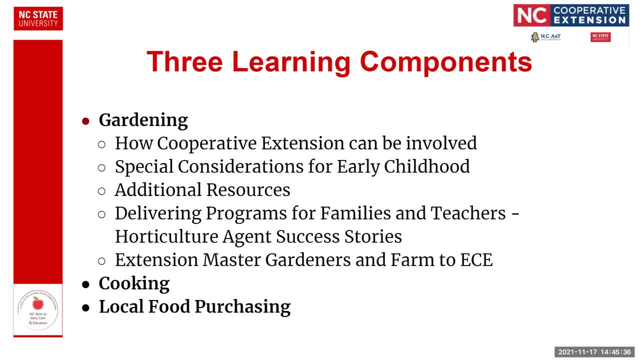 This isn't necessarily like new, all new, brand new information for agents, but more like you know, a depository of where can you go for this, Where can you go for that? A lot of that already exists. So we're not trying to recreate the wheel, but just kind of have a place where agents can go and say: OK, I want to do farm to ETE. 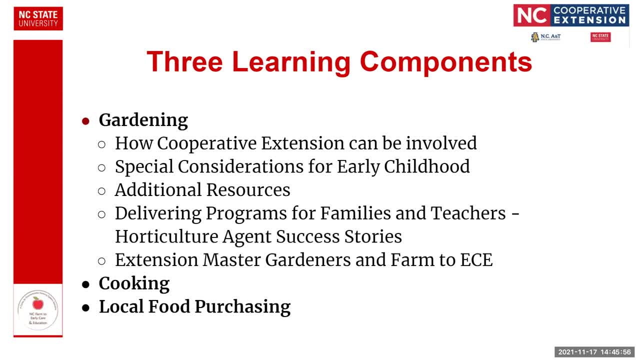 I want to focus on this And then this is where I can go to kind of make that happen. We have some success stories in each of these areas And then we have different, different extension programs that folks can plug into. So, of course, for gardening, that extension, master gardeners. 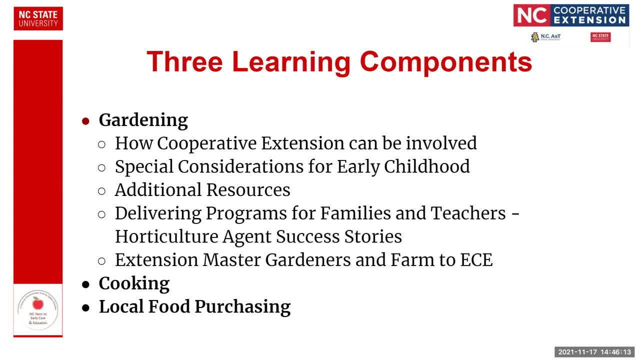 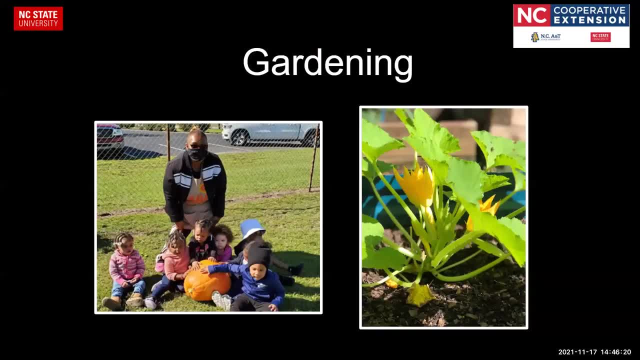 And then for cooking, we have the master food volunteers, That kind of thing. So for gardening, of course, we have to include as many photos of adorable young children playing in gardens and with garden produce. So check, Aren't they perfect? 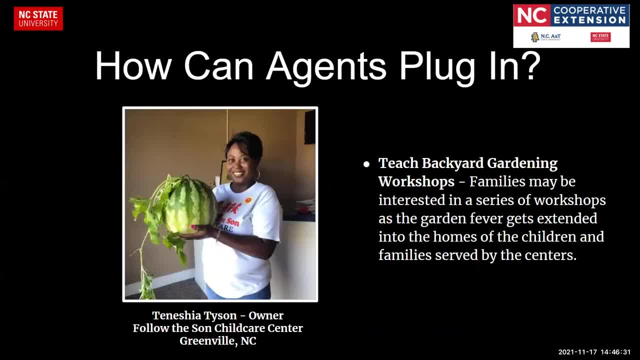 This is a center in Greenville, North Carolina. I've just harvested their pumpkin. This is our friend Tanisha. I follow this on Child Care in Greenville. So our first section in gardening is: how can agents plug in? So I have just a couple of examples. 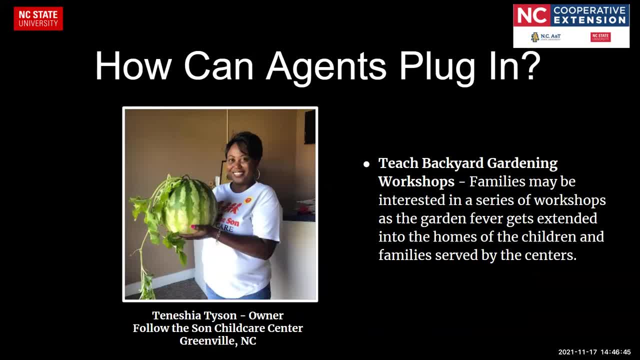 Pulled from our guide. this is not all of them, But, just as an example, a lot of agents are already teaching backyard gardening workshops. We'll invite families from child care centers that you can work with, Right. So expanding to new populations, inviting, you know, not working necessarily harder, but smarter. 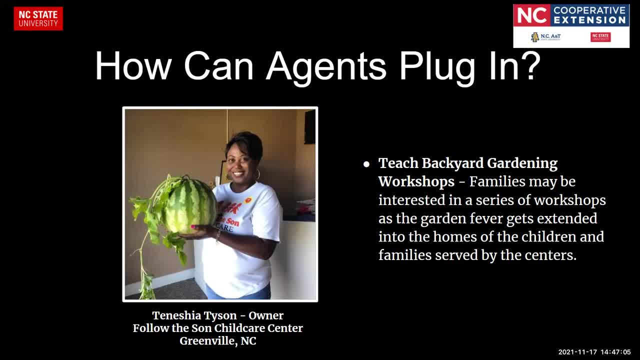 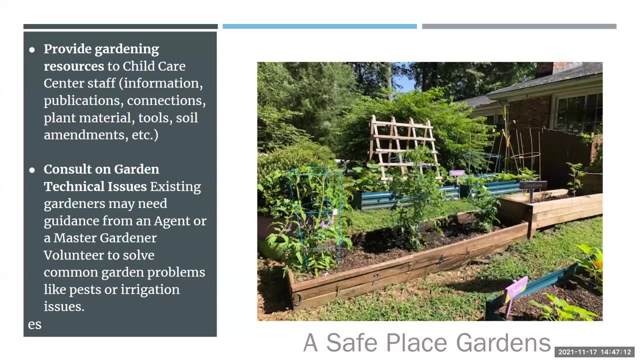 Right Inviting these folks in the workshops that already exist. Center directors can also join. join those workshops A lot of center staff once they get going with their gardens. they're going to need that consultation on gardening technical issues. They're going to need those resources. 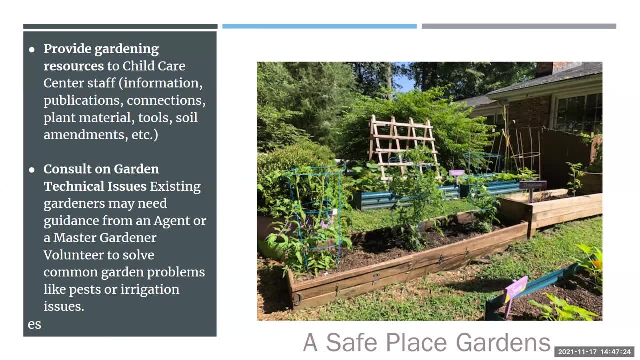 And so this is such a great way for master gardeners to plug in. Maybe they don't like working with children directly, but they really like working with adults and gardening. This would be a really good opportunity for master gardeners and for horticulture as well. 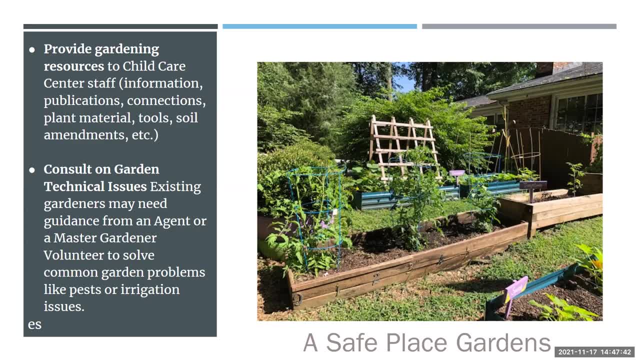 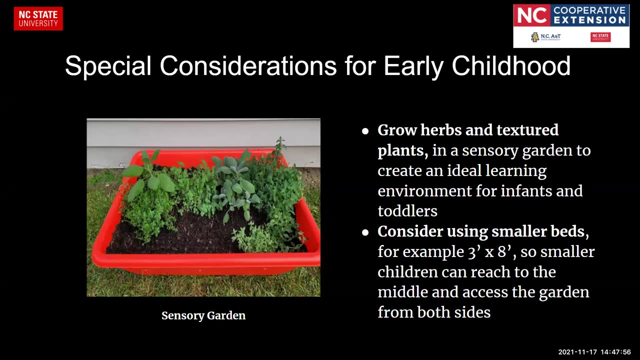 So this is actually A safe place. So I correct me if I'm wrong, but I think it allows a lot of work with this garden in particular, And you can tell it looks really beautiful. Yeah, So cool. And then the next section in gardening, and on all the sections, is special considerations for early childhood. 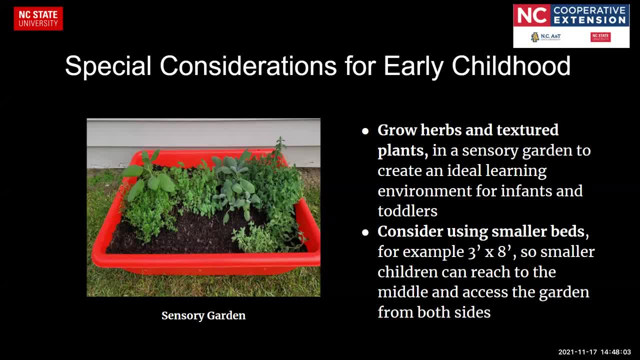 So folks that are new to working with young children, are kind of new to early care and education environments- can know a little bit more about it. can be a little less intimidating, Hopefully, To have some of this background knowledge about how to work with children. 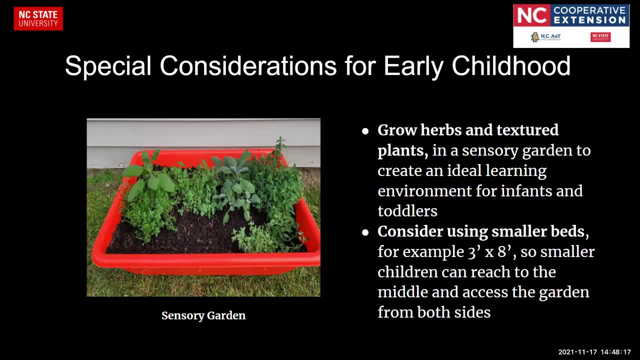 So some special considerations for early childhood in the garden, of course, you know, considering those smaller beds so that they can reach their, their tiny arms in the middle. for both sides, That might be one that's kind of obvious to to horticulture agents. but then, thinking about from the early childhood perspective, teachers love to get children around learning about their different senses. 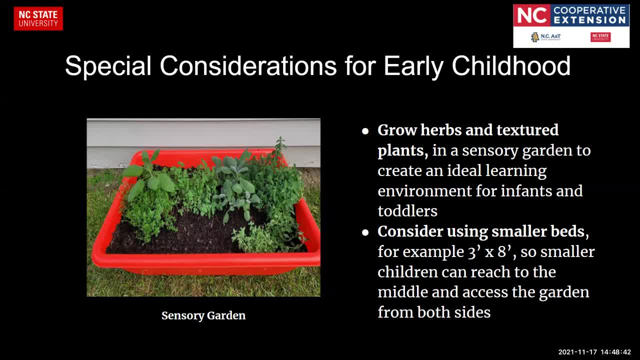 Like it's really cool, Cause it's it's Age, like everything is so brand new to them, Right? And so one thing that we love to do with really, really tiny children, like infants, toddlers, is to have them in those sensory gardens where they can smell, they can touch. they can- don't let me maybe name all five, but you know they can. they're like listening. 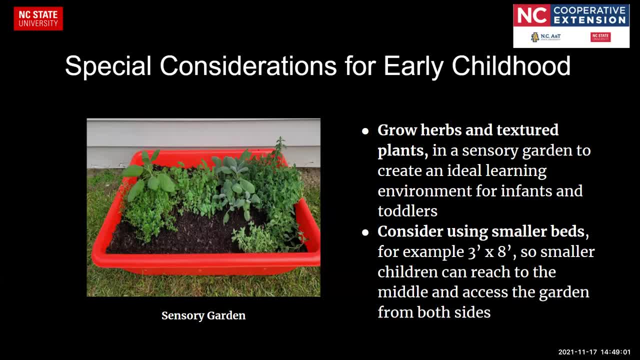 Maybe there's a little water source or you can hear these, you know that kind of thing where teachers can can use the garden to teach, Right? That's what it's all about, And then just to touch on the Other two content areas really quickly: 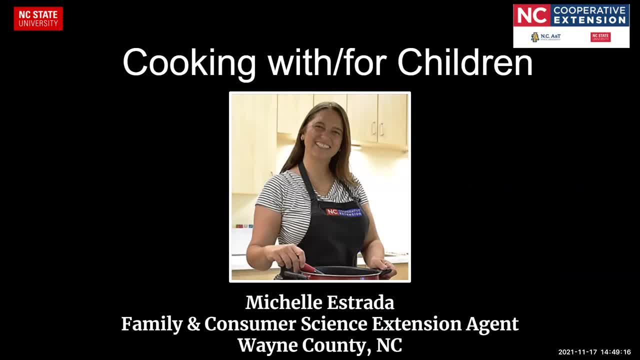 Um, so cooking with children and for children. so our family consumer science agents love doing this, because it's not just about, um, you know, doing the taste test in the classroom with children, which is awesome, you know, promoting that local food. 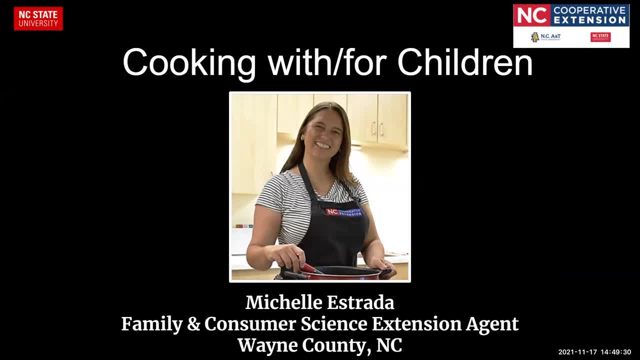 And I- um, you guys probably have heard of that, but it's also about, you know, working with those cooks. How can we get them excited about using local food in the kitchen? You know, maybe it's new to them. 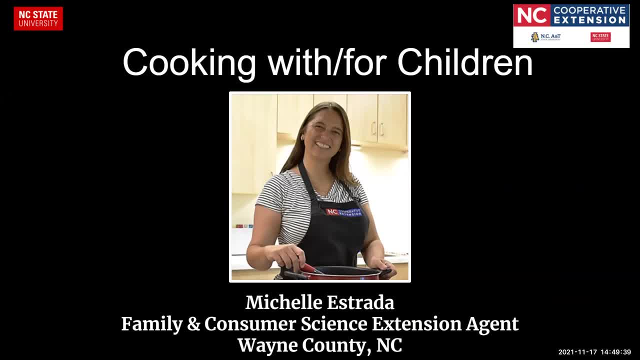 Um, but they're already doing. you know some, uh some, nutrition Work Shops, cooking workshops. You know how can we pull in those cooks from the early childhood community to really join that um and promote that here? 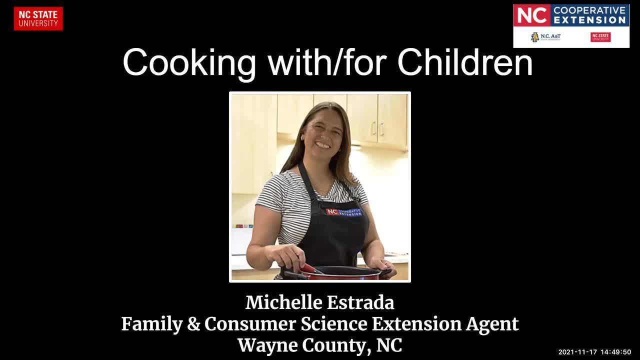 So I've highlighted one of our star agents who, um, who's also going to review this, but I don't know if she knows it yet, but, um, her name is Michelle Estrada and she's just wonderful. She's done a lot of workshops for us and um and our ECE providers. 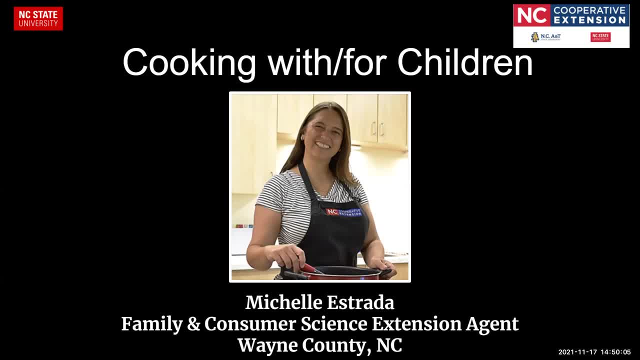 And, um, she also used to be a preschool teacher, but you do not have to have a huge knowledge of preschool to do this, but it does kind of help That she, um, you know, has that background, of course. 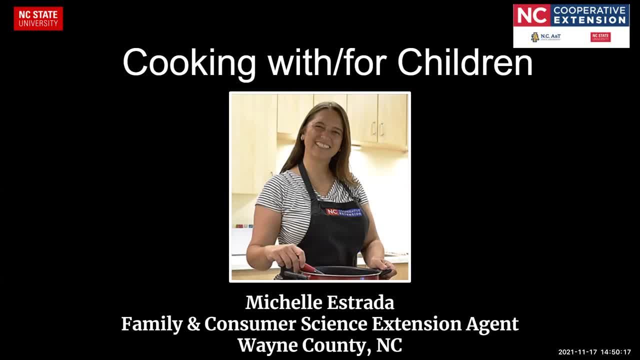 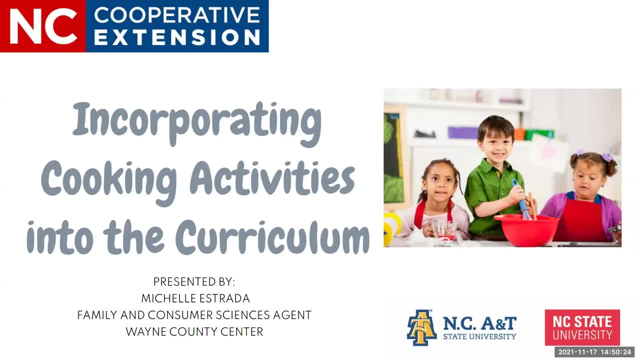 Um. so she has done some virtual stuff for us. I have here, um, just the title side of one of her, her virtual opportunities for our teachers from across North Carolina. Um, it's called incorporating cookies cooking activities into the curriculum. 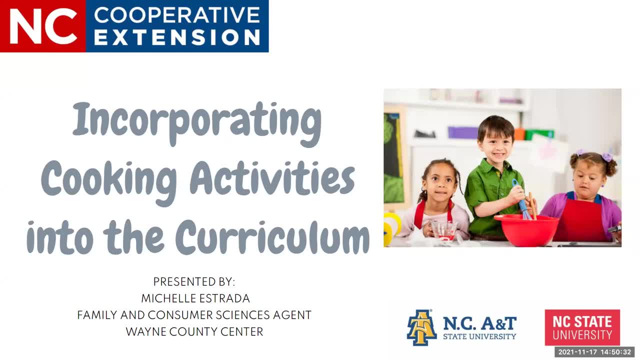 So she does, you know, a few sample recipes and then she, you know, asks the providers to talk about: well, how can you incorporate this into STEM or into arts or that kind of thing? Um, but really beautiful opportunity For SPS agents and farm TV. 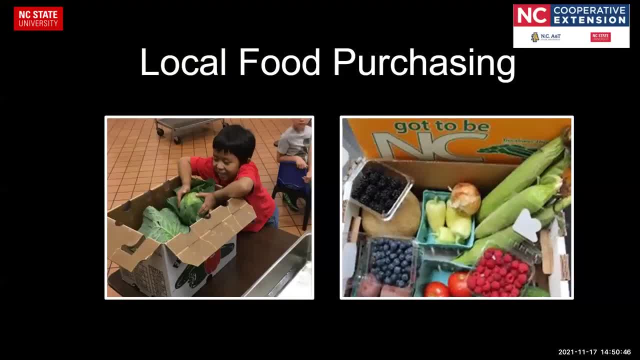 And then, lastly, our local food purchasing. So um ag and hard agents have been really helpful in connecting farmers to um the early childhood community, And so right now we're still trying to figure out, you know, the most um viable ways to do this for farmers, so that it's not um necessarily something that they're doing. 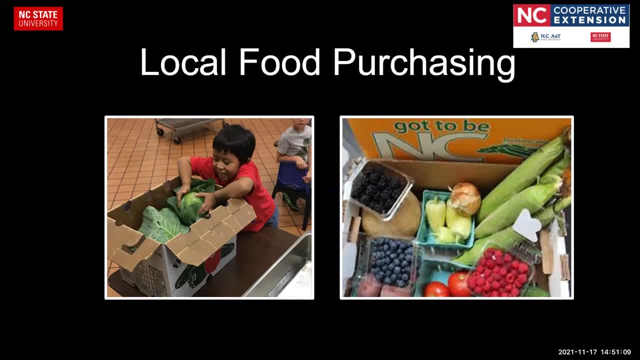 I guess I should. let's see how we're trying to make sure that it's a viable solution for farmers and for the early childhood communities. right, because right now, um, we found that, like csa boxes are a really good way to do that- local food purchasing but other direct farmer 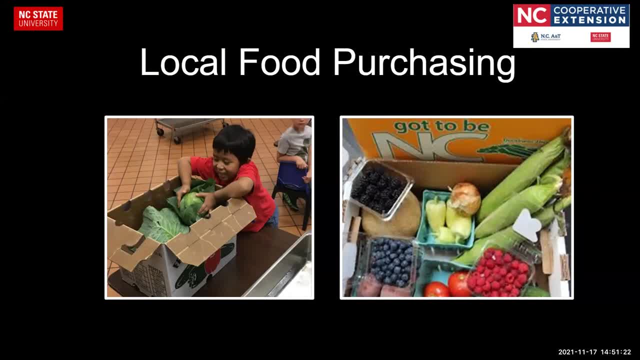 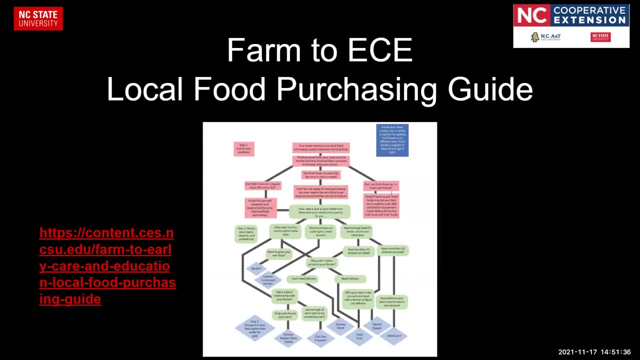 sales. um, it seems to really benefit the child care center. um, we're still working on how to make sure that that benefits the farmers, but, um, it looks different in every community, and so, um, we have a guide here that we've already created, so this is a the new guide, but it's referenced in 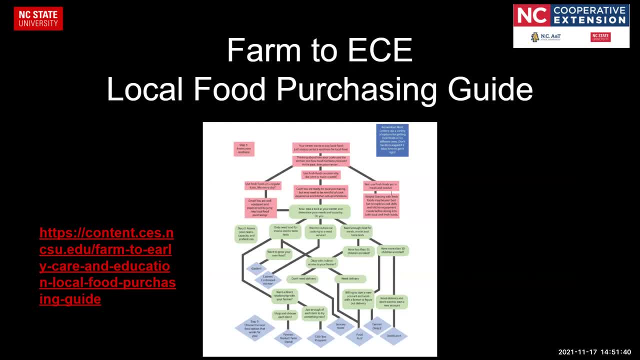 our new guide. um, this section is pretty much pulling a little bit from this local food purchasing guide, which is also on the website that lucy shared. but, um, this is a decision tree so that if agents or technical assistance providers want to work with the director and 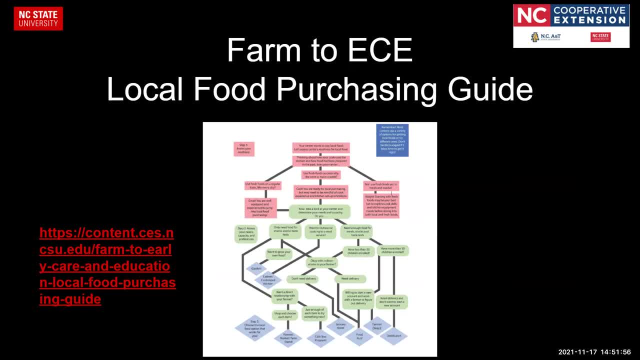 how they purchase food. they kind of start with like, okay, what is your goal for local food purchasing? is it, to you know, connect with a farmer and have that relationship? is it to get as much local food as you can? that kind of thing, and it goes through this decision. 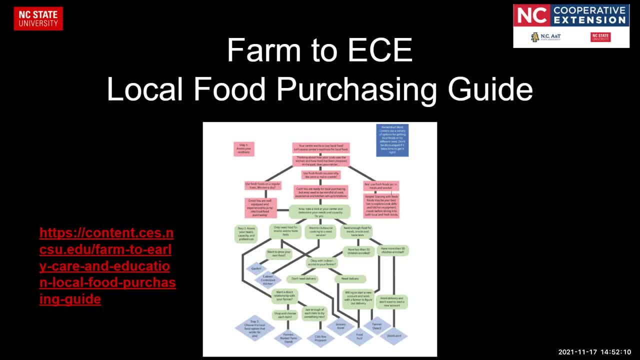 tree to kind of say: oh, if you um want to do a, b and c, then the best local food option for you is to go to your local grocery store, ask them, um you know, for their local food, that kind of thing. um call your call cisco, and say, hey, what do you have up? local that kind of thing. um, so that's a. 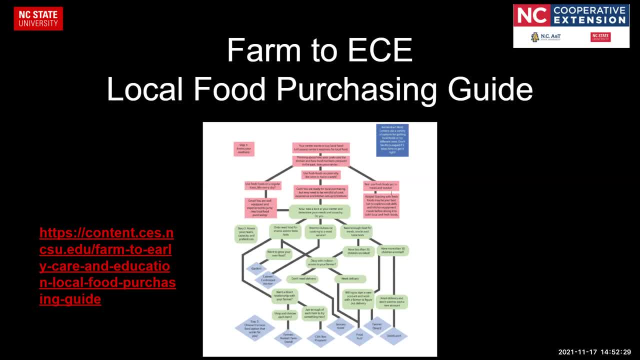 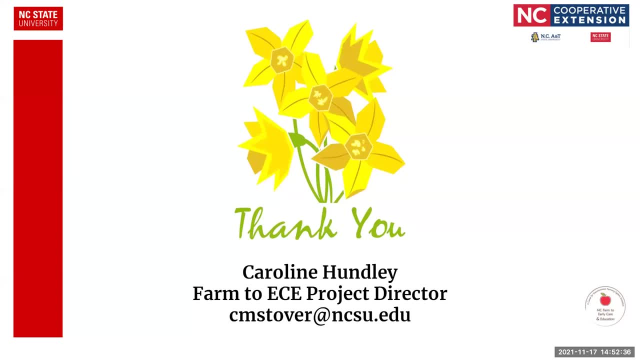 tool that we have to help folks really um purchase local food. so that was kind of a rundown of what we um have outlined for the guide so far. i would love to hear any questions, feedback, ideas that you guys have. like i said, it is not um, i'd say it's like 95 there. i'm so excited for it to be done and reviewed and 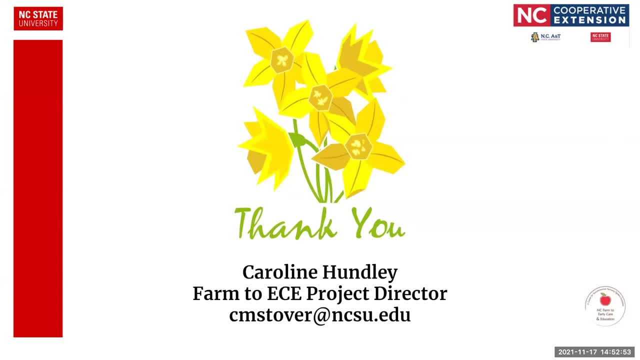 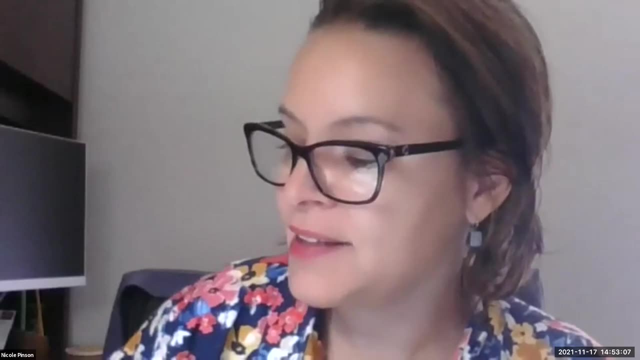 on our website and we'll certainly be in touch when it is thank you. thank you, caroline, and thank you, bria um and also lucy for posting all of the resources in the chat. um, i have a few comments and i i do. i did see in the chat that some folks were mentioning how happy they are that you included. 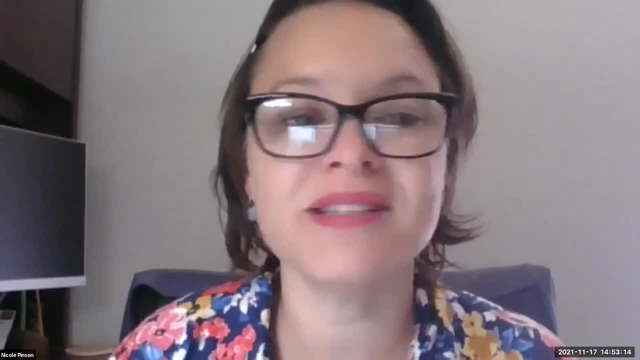 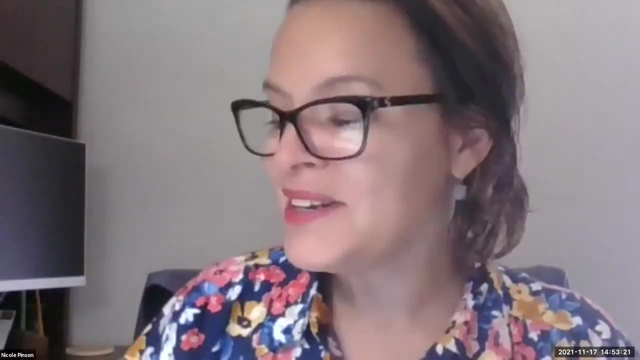 arid plants in the west, uh, so i guess that's sort of an underrepresented area, so they're thankful for that. um, i was thinking of ways that i could use this and it was pretty. and it was pretty exciting because i'm looking at the activities and i thought, first and foremost, a lot of them. 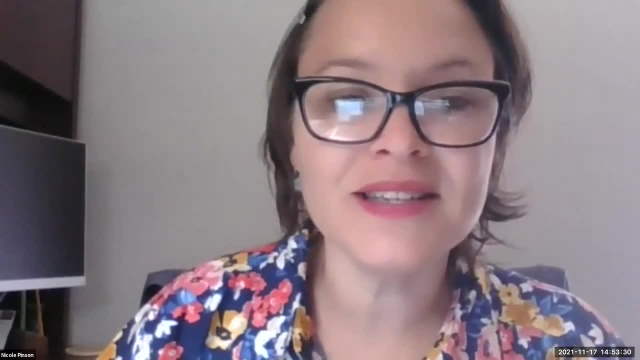 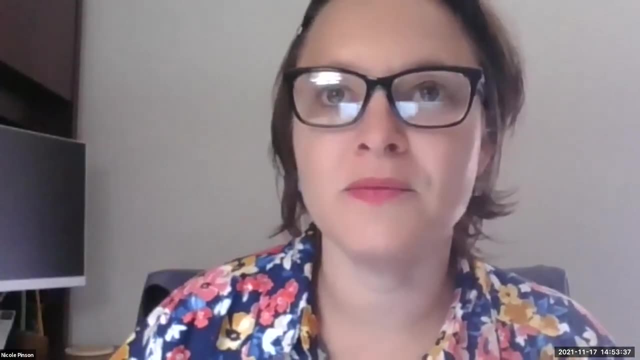 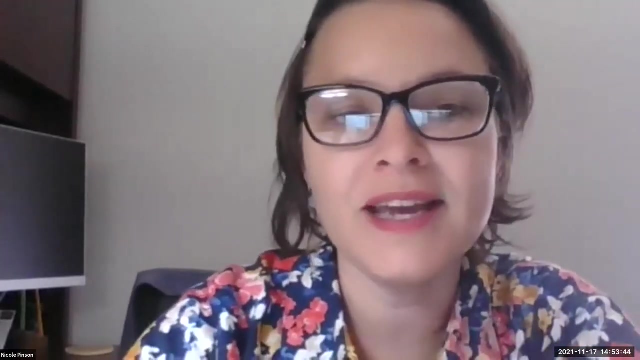 were really fun, you know, like making leaf necklaces and the activity eating and sharing. i could see doing this with kids. um, i know, in extension sometimes develop different programs and we sort of start from scratch. but you all have packaged this so well that people can, um, you know, sort of just take these activities and adapt them into different. 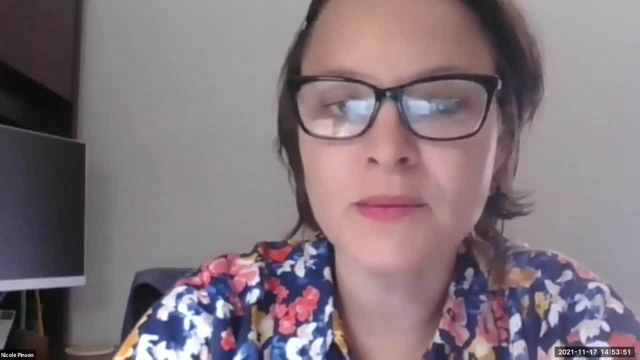 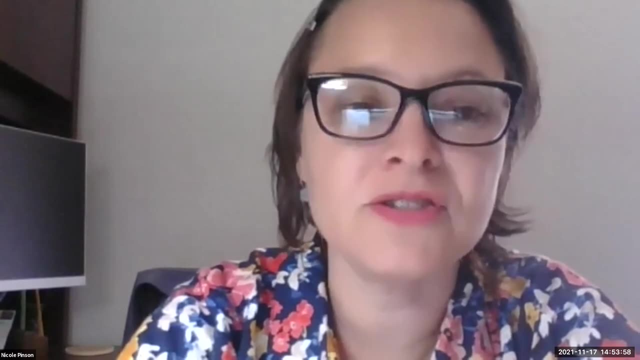 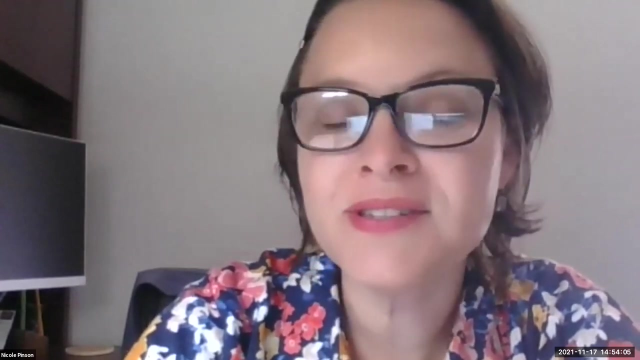 programs like school and community gardens. i could see this with some of our homeschool groups in florida and even, as you mentioned, collaborating with agents, fcs agents, 4-h folks, so they're really interesting activities for kids. i love that the pictures are, you know, just kids out gardening and it's not, you know, like pinterest worthy pictures. 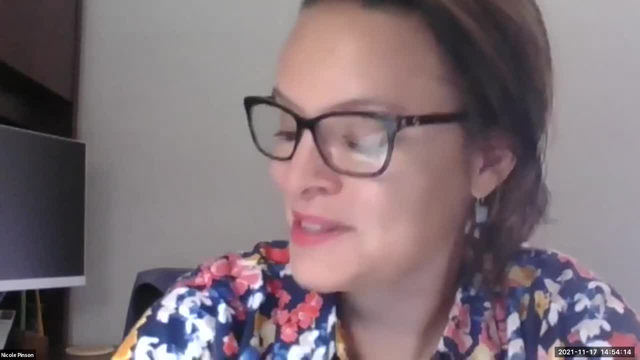 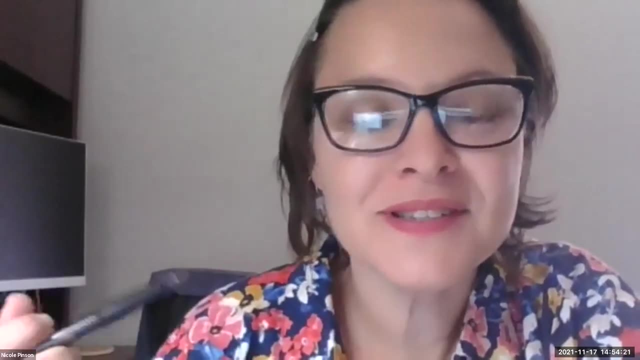 everything just looks like you would have if you're working with um a bunch of kids and they look fun. and something else i thought about is: you know, we tend to write articles as, as extension, people and in horticulture, and i don't often write a lot of articles that could be directed. 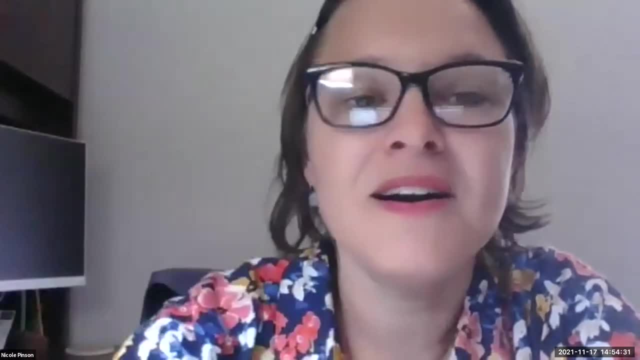 to parents and children with gardening, and so that made me think, uh, maybe identify some of these activities, write some articles for parents, and i think that's a really good way to do that. so i'm going to look that up and probably link to that, just to kind of give the parents and kids. 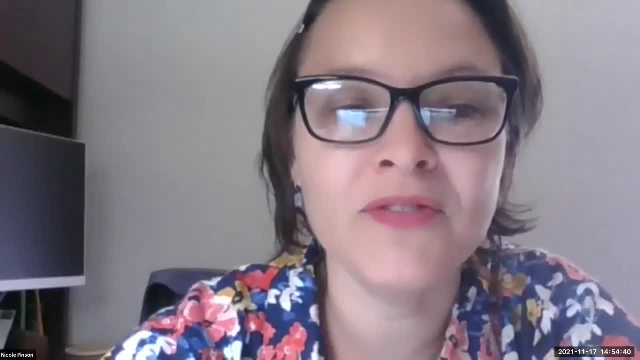 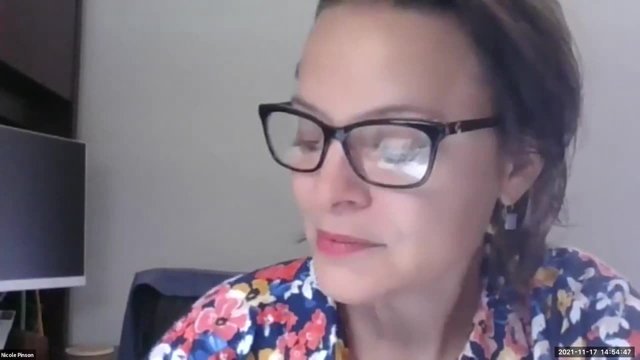 or grandparents, and we could hyperlink to your website where people can find more information and other activities to do so. that got me thinking, because i'm actually writing an article right now about native native plants and how they attract birds, and which ones would be great for florida. 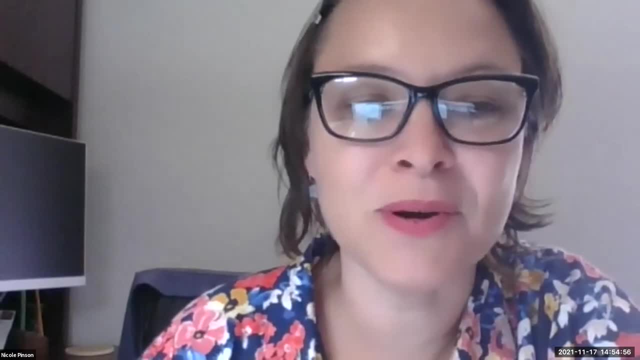 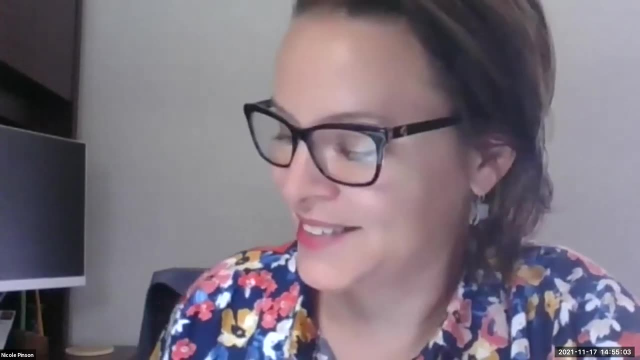 but i noticed that you have a child's activity- birds and bird habitats- so i'm going to look that up and probably link to that um, just to kind of give the parents and kids something to do. so for those of you who are interested in gardening and kids or grandparents and kids or grandparents- 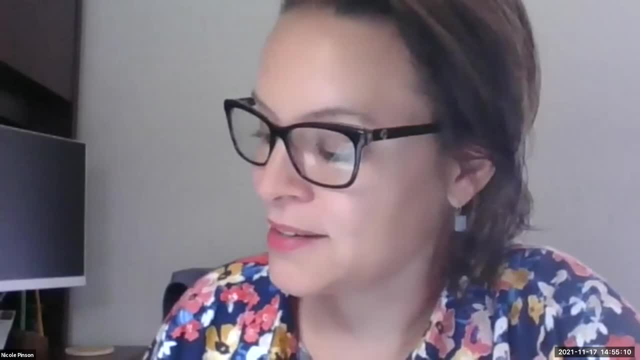 i'm going to link to that as well. so i'm going to link to that as well. so i'm going to link to that as well. so, for those of you on the webinar, feel free to unmute your mics. ask questions, put them in the 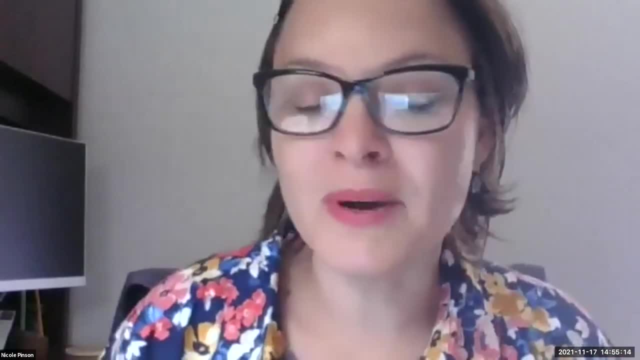 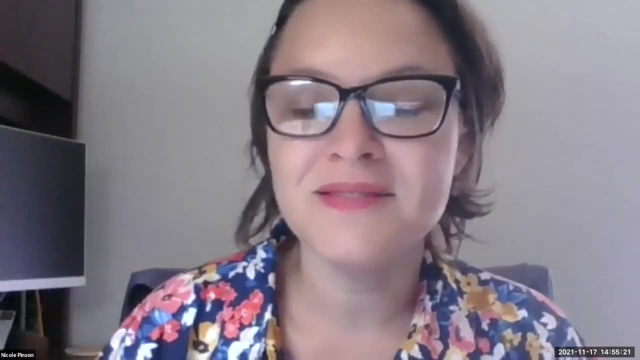 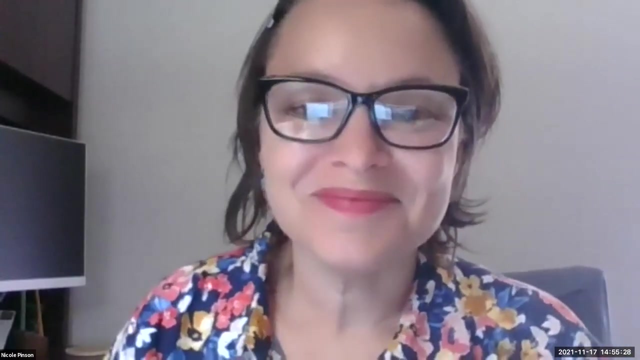 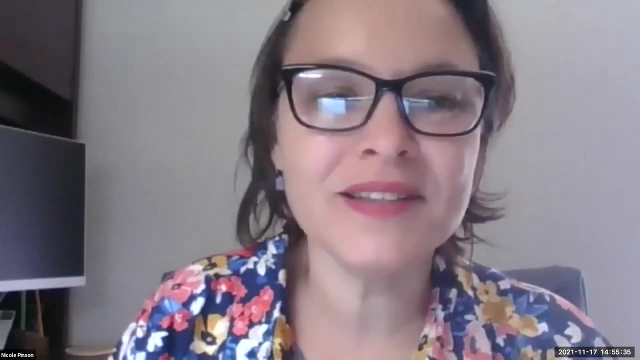 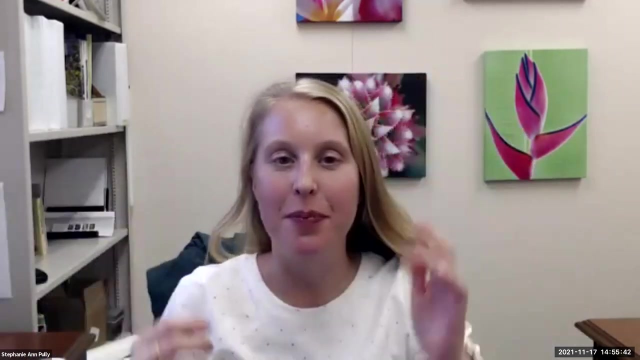 chat box. um, these are excellent resources, and what i love about north carolina is everything is always so well packaged, easy to understand, user friendly. it's all great. do we have any questions or comments from the folks on the webinar today? i have a question. yes, hi, this is steph. i'm the state coordinator from maryland. um, i was just. 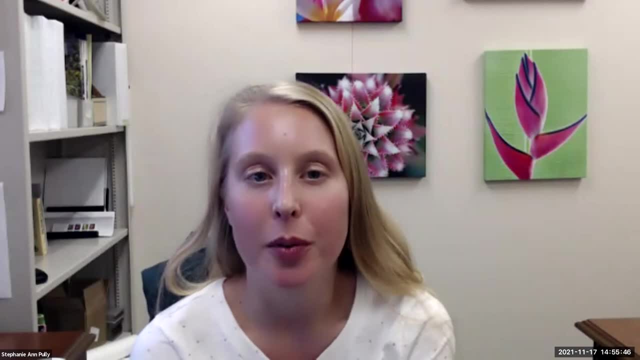 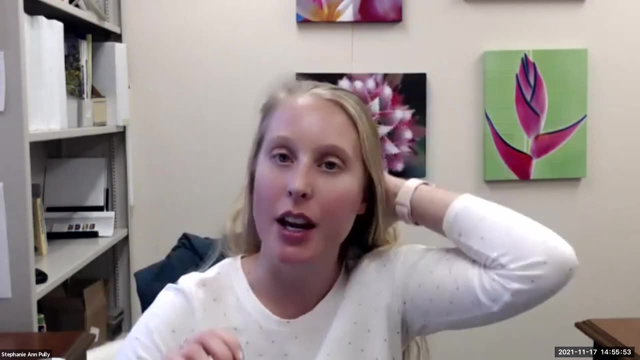 wondering: how do you get your volunteers to be comfortable working with children? because i think that's a hesitation that a lot of people have. you know, they weren't like formally trained in any type of child care or education and i think they just get concerned about all the liability that goes. 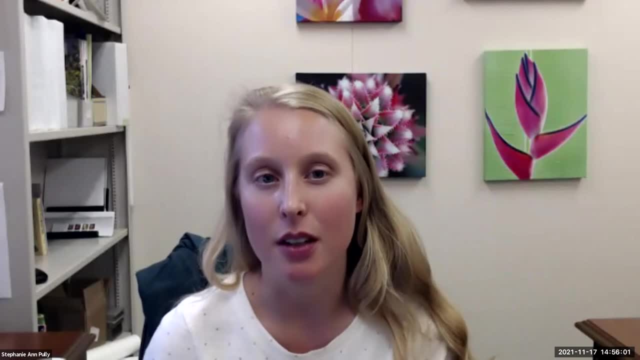 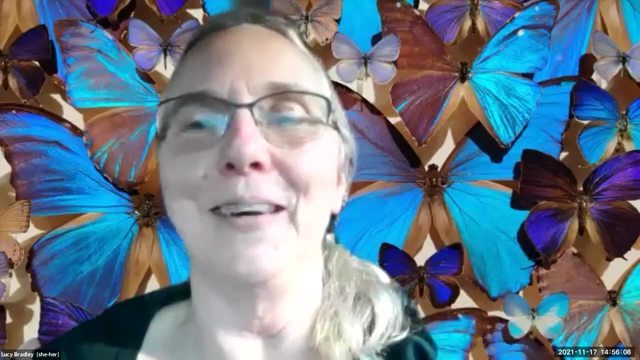 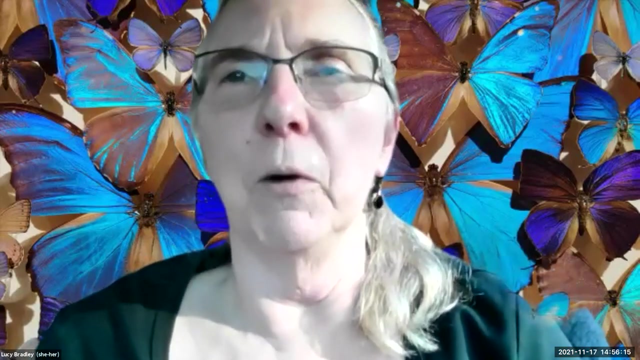 along with working with children. so how were you able to get volunteers to be comfortable with that? i might welcome charlotte's input into answering that question. stephanie, um, we tend to have people who are interested in working with children. one of our challenges is: is the liability and figuring? 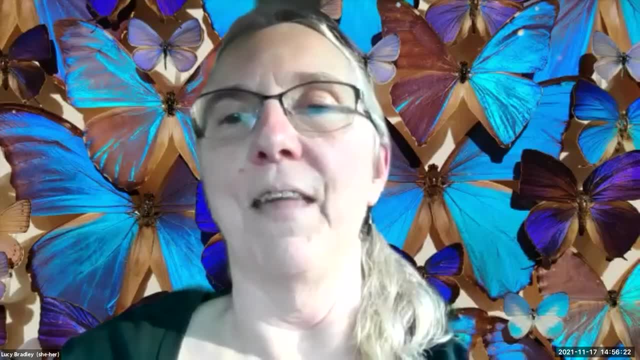 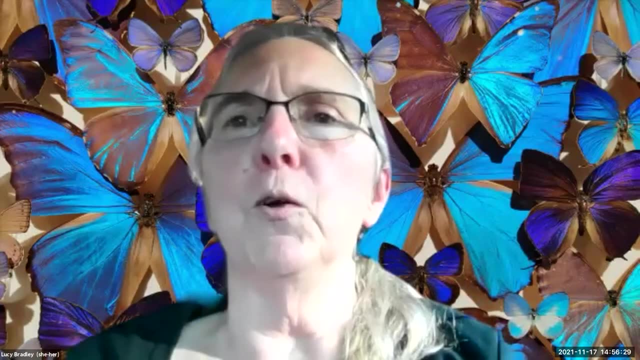 out. you know who needs to be fingerprinted and and how that's going to work, and we we've- i think we pretty much- sorted that out so that we're ready to go. um, these are really designed for people, who, who want to do it, so who who are approached by preschools, who want to do it and who and who have. 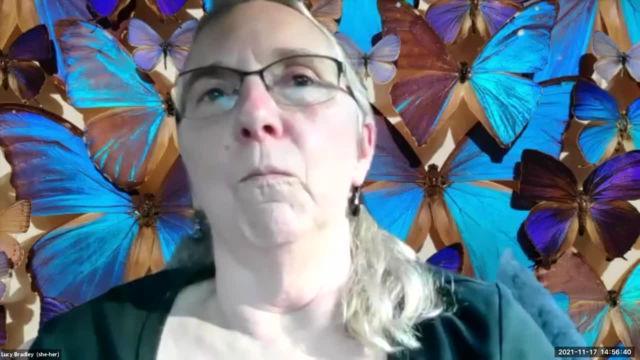 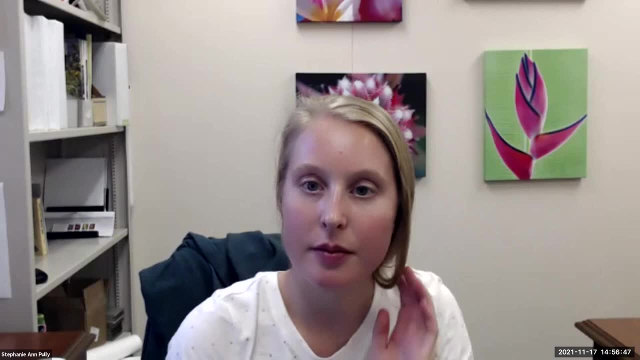 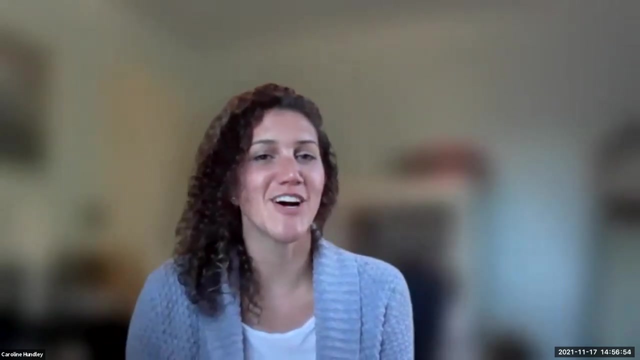 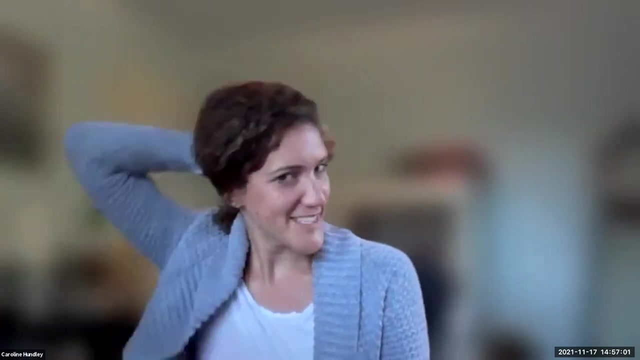 been doing it for years and want to jump in. this is like: how do you do it? okay, got it, thank you. i don't run the master garden program at all, but i. what i also love is that there's so many opportunities for folks that don't necessarily want to work with children like even: um, it's kind. 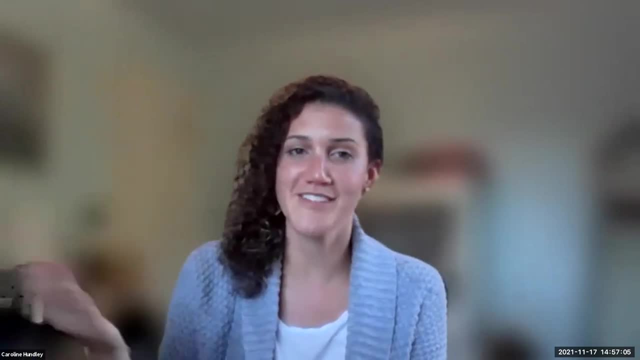 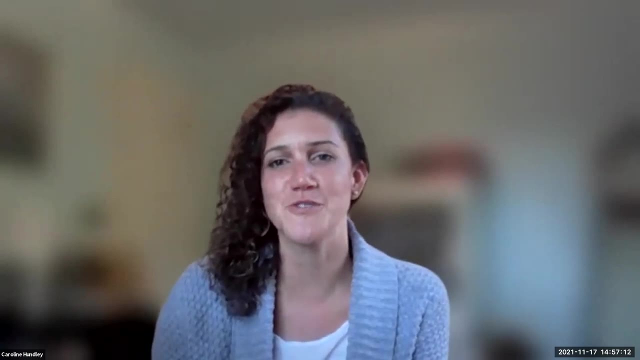 of similar for our child care teachers, like if they don't want to work in the garden, well, you can write the newsletter. like you know you can do something else that's related. so i think too, just maybe just embracing, that not everybody wants to work with children, but they can still support the mission. this is tracy from delaware. 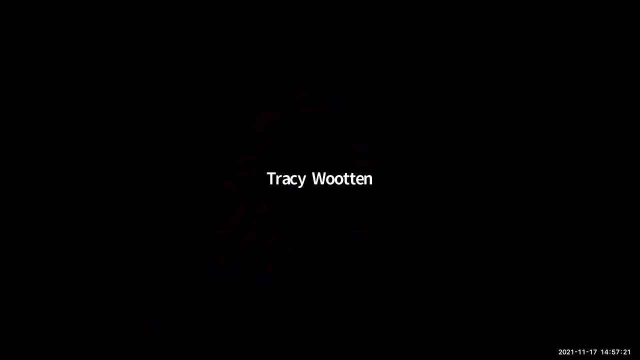 and definitely we make sure that everybody's got their. you know background check and that kind of thing. but i we have only three counties, but each county has their own personality and i know here in sussex, you know, i have so many people that are retired teachers and just don't. 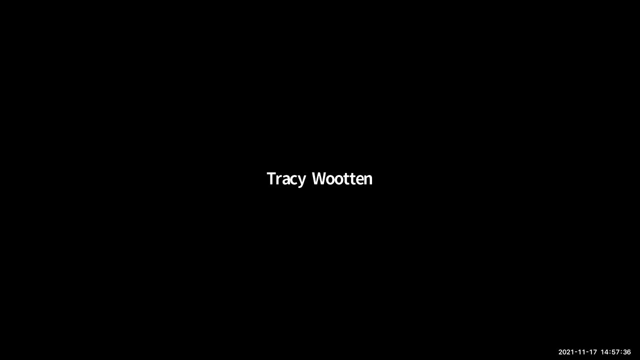 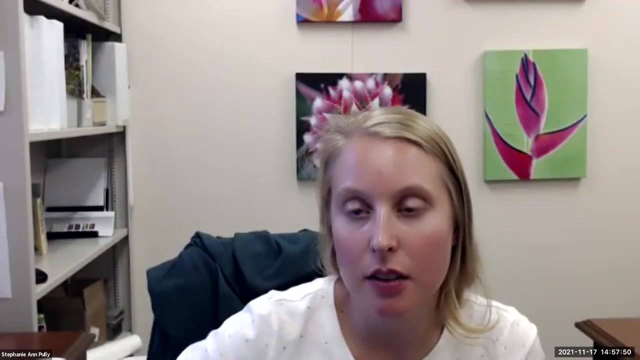 you know, just so enthusiastic about reaching out to children and youth, so we've really developed people in our organization that have those skills to help mentor others, and that's been a huge help as well. yeah, the mentorship is a great idea. yeah, i mean, we even in our demonstration garden we have a whole children's garden. 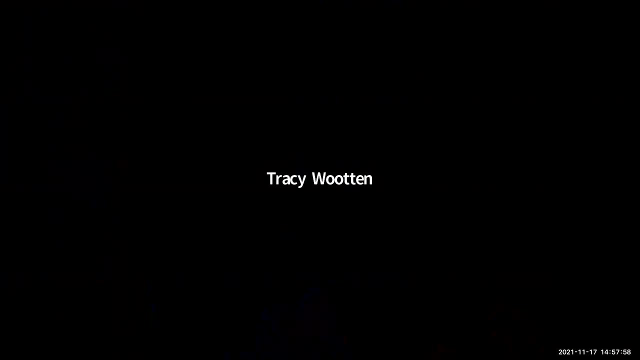 we have a lot of things and again relying on that creativity of your volunteers. um, we're just going through training right now. we just had presentations from our trainees and just i'm just just seeing how this can be with the kids from our trainees and just identifying who has that interest and skill before they even get out. 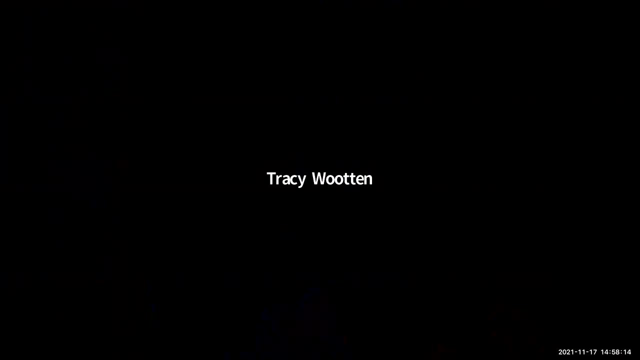 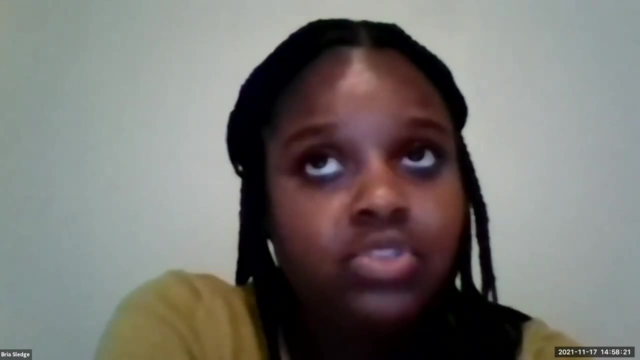 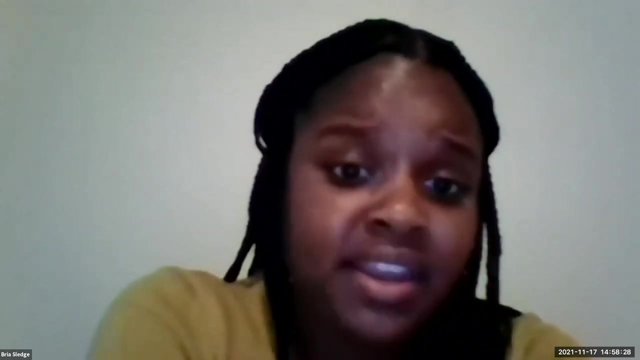 and start volunteering is has been very helpful, awesome, uh, i can add to that. i can't really touch on volunteers outside of the child care centers or school, but what we try to encourage is maybe identifying a staff member that's already working there, who loves to garden and what is. 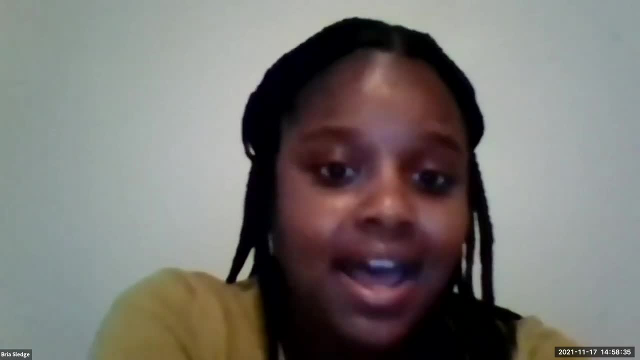 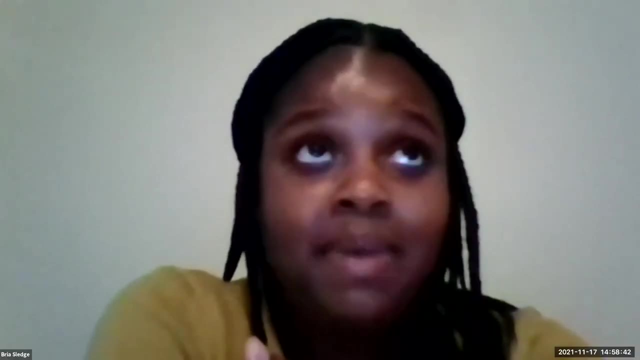 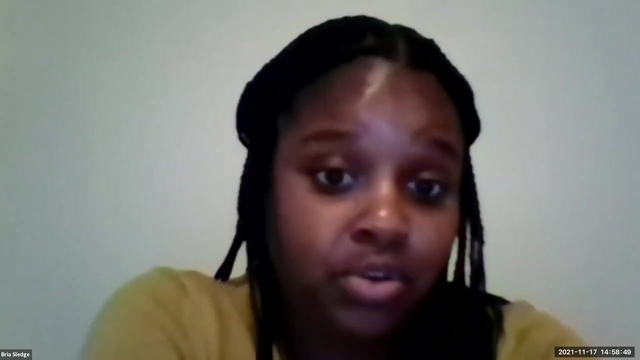 willing to pick up that, um, that task at the child care center. it could also be talking to the parents that you have a wealth of different parents with different backgrounds who specialize in different things, or you have kids that go there, so it could be a landscaper who is willing to come and spend. 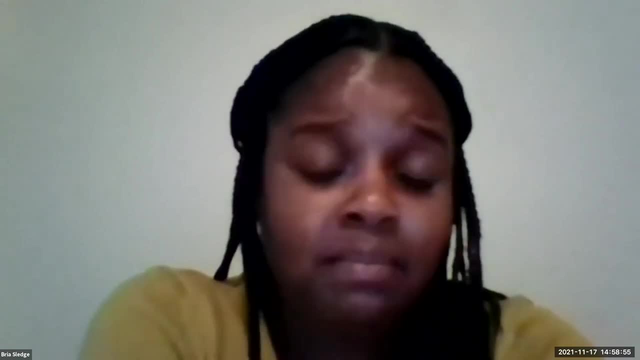 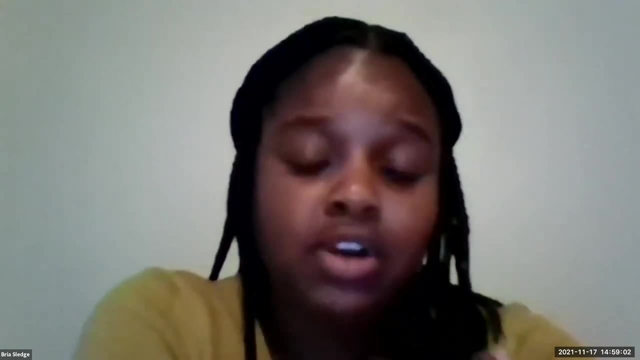 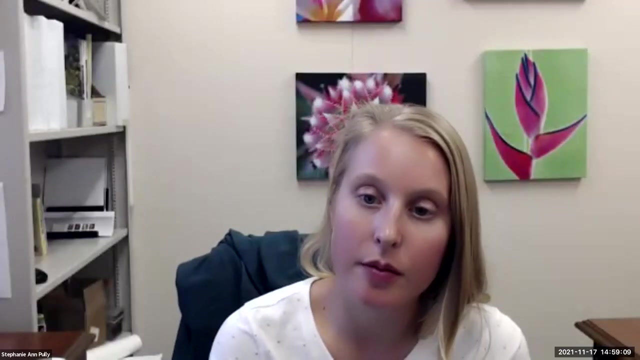 some hours working on the outdoor environment or maybe donating some things. um that, um, it's necessary to make sure that those um plants grow. i mean because the child care center- they are specialized in working with young children and making sure that they're educating them and that they're safe, so that's their top priority. but 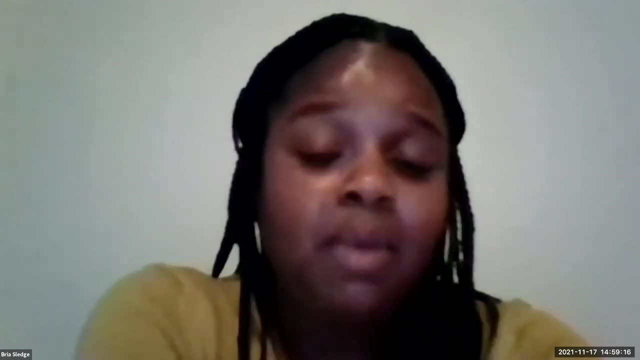 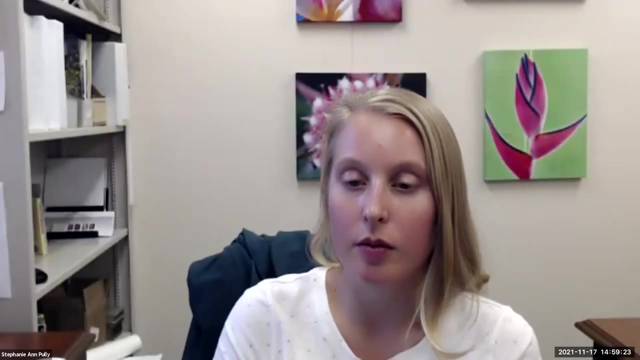 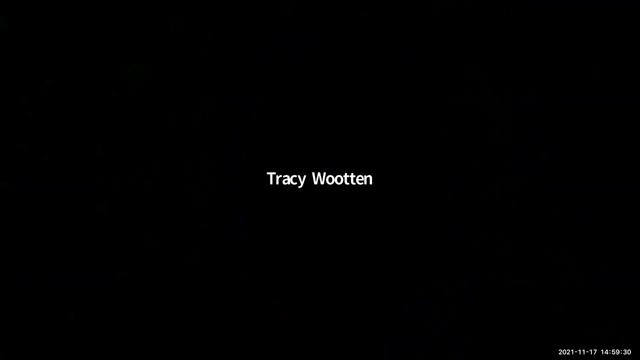 we want to make sure that they're thinking outside of the box and using the resources, tools and professionals that are around them. um, to make sure that that's possible. um- and i'll also jump back in and say that- um, for our community and school garden programs. we go across program areas and we've actually started training kind of hybrid uh volunteers who are looking at health and wellness, um and pairing with master gardeners so that they have both sides of that. you know, you have the nutrition aspect with the schools, um and communities as well. 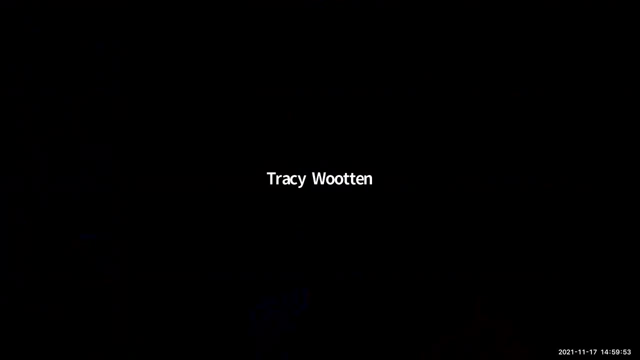 as the technical piece with master gardeners. so that's been a unique thing that we just started in the last year and that's been good for being that- that person that interacts with the schools, um, but it is a lot of coordination and making sure everybody's on the same page in all different areas. so 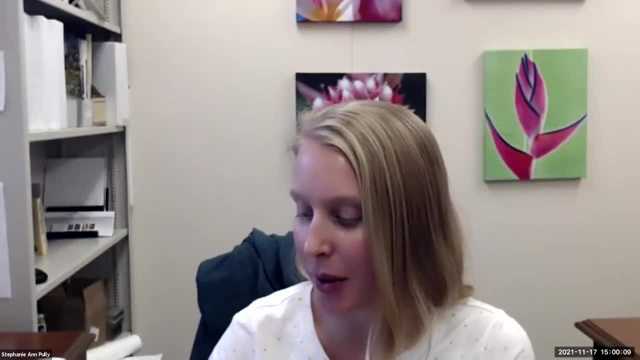 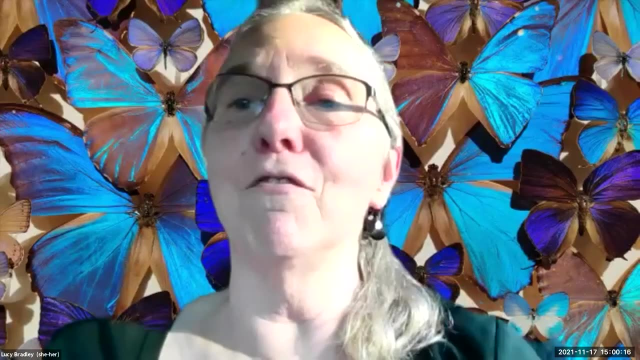 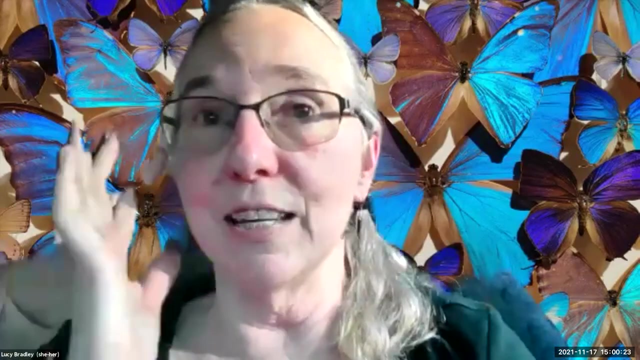 but it has been. i mean, i love the partnership, though, and it just makes a lot of sense. i think master gardeners, many of them have grandchildren who are preschoolers, and and many of those grandchildren are on the other side of the country, so they're tied in and interested. 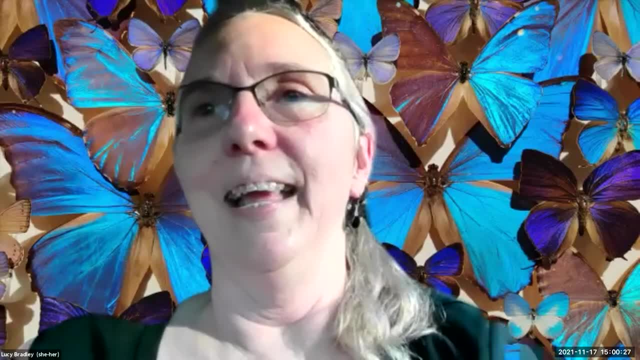 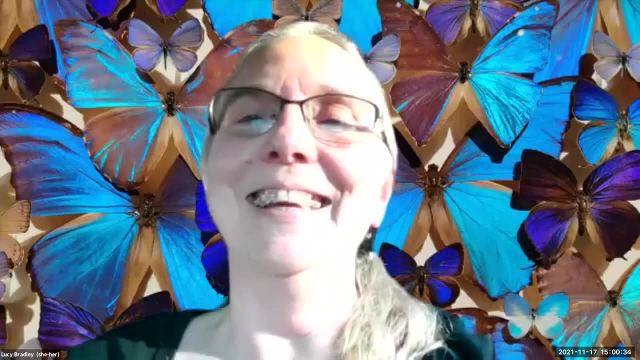 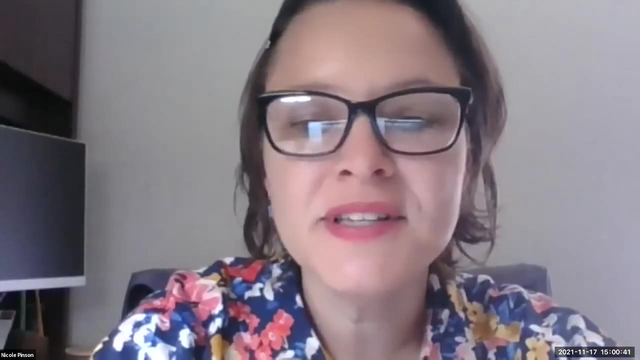 in um working with young children, you know whether, as you know, kind of surrogate opportunity or practicing before their children come visit. and another way um we could use the activities that you've put together is, if we have extension demonstration gardens, taking a look at the activities and seeing if there's some that 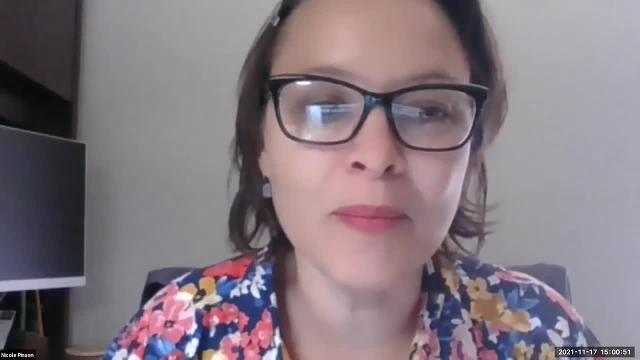 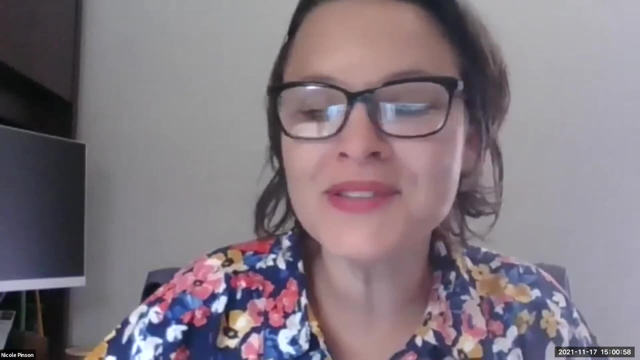 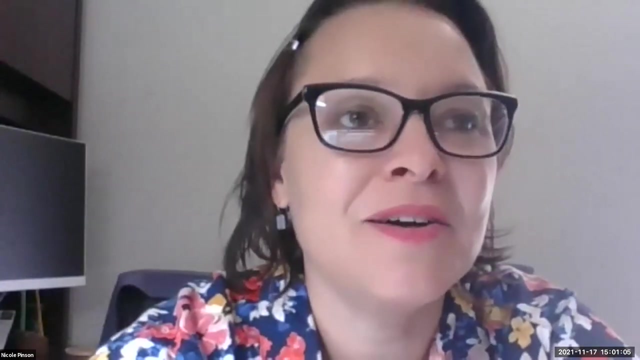 we could integrate into our existing garden. so i saw a very simple concept called pebble play and that caught my eye because i've never seen that before and you can easily arrange a few pebbles in a section of your extension, demonstration voilà garden And then, when you have families and groups visiting, you've got some little things that can. 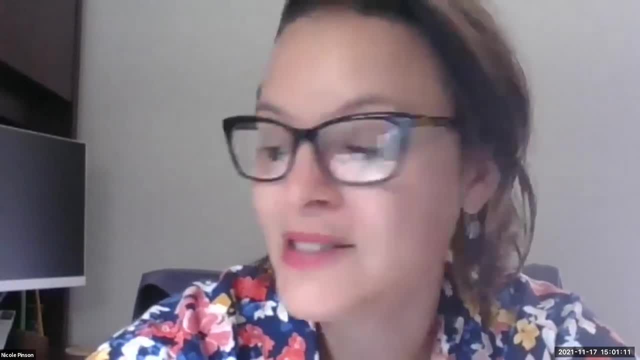 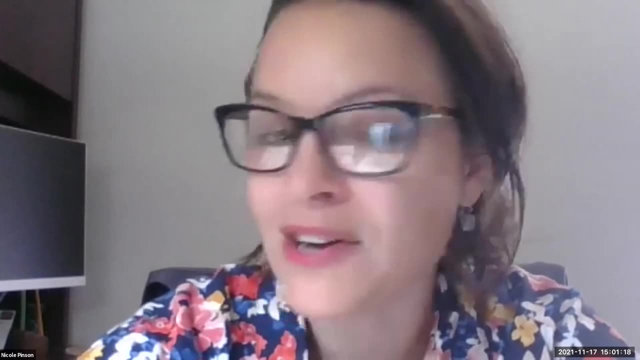 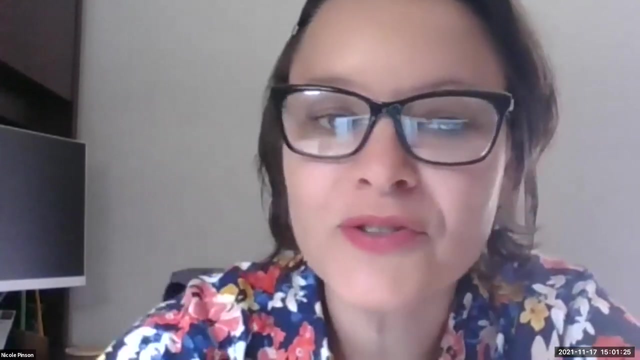 get the kids engaged. So there's a lot of ways to use these And I don't know, even like Great American Teach-In, but I just I find it just wonderful activities and a lot of fun to get kids engaged. Any other questions or comments? I do see a comment in the chat box from Colorado that 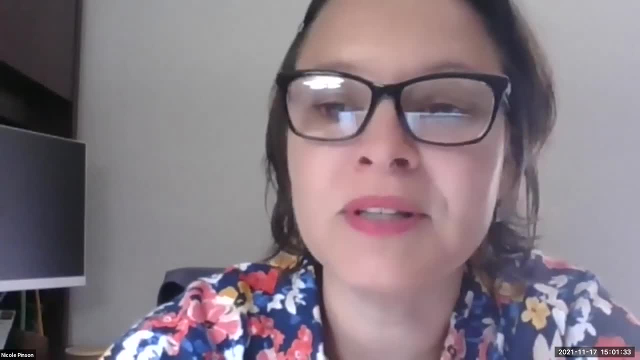 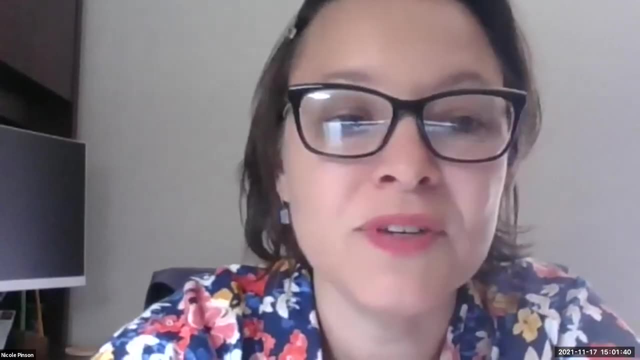 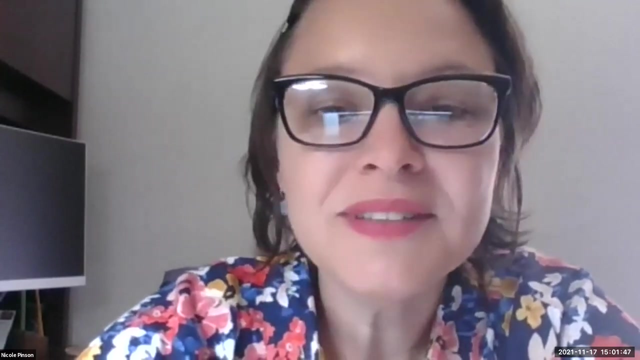 opting in, not opting out, is important when working with special populations, And I would agree with that. That goes, you know, back to recruitment and matching people up to the best fit for your volunteer program. Well, hearing no other comments or questions, of course, if you do. 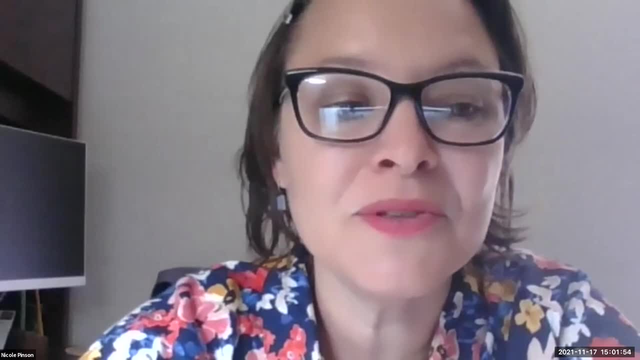 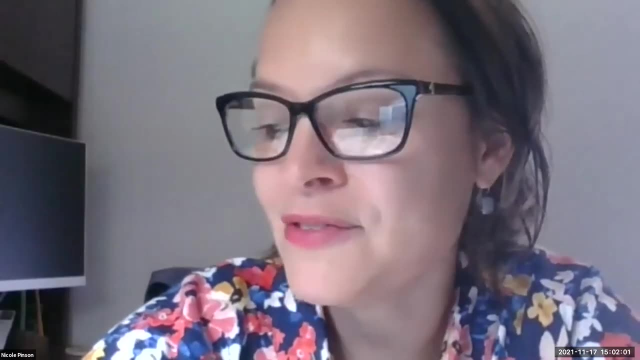 have some go ahead and put them in the chat, But this was an excellent presentation from the three of you. Thank you so much, Caroline and Bria and Dr Bradley, for speaking with us And giving us some ideas of great activities that we can do with youth- not have to reinvent the. 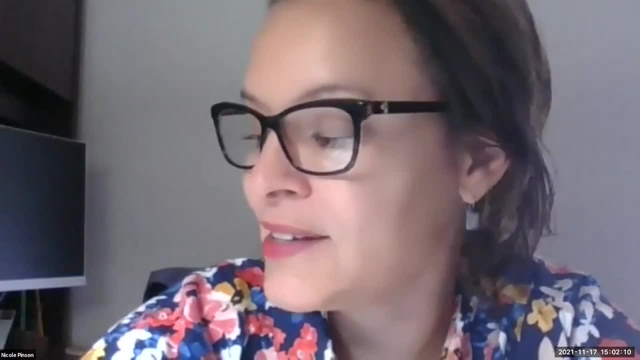 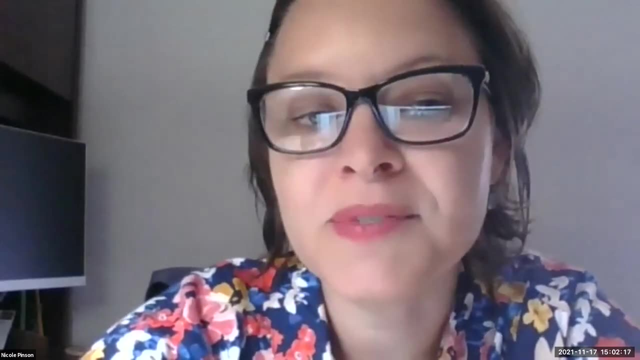 wheel, use the resources that you've graciously shared across the country and, you know, possibly collaborate and link up with our colleagues to do some of these programs that are across departments or program areas. So, thank you all so much. If you want to reach out to our speakers, 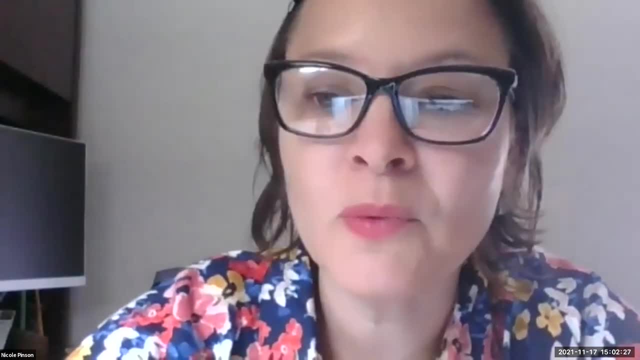 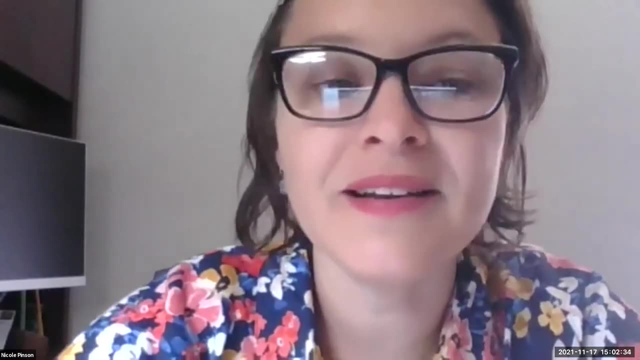 we'll send out their email and contact information. We'll post a recording of the webinar And also follow up with some of the links that were shared today. So thanks everyone for being here And I hope you have a good rest of your week. Thank you again, Lucy, Bria and Caroline. 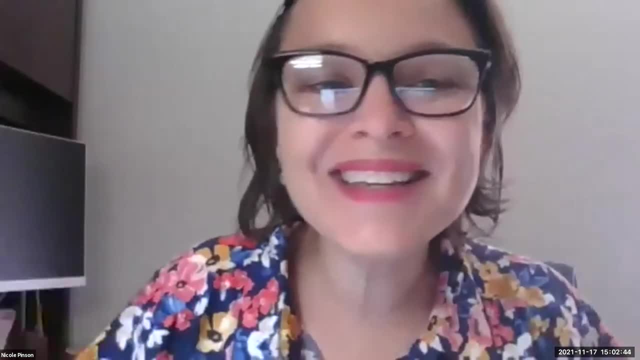 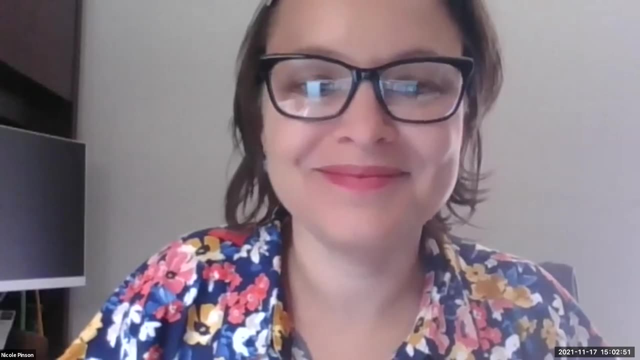 Thank you. Happy Thanksgiving everybody. Yes, happy Thanksgiving, Take care Bye, Thank you, Bye-bye, Bye, Bye.